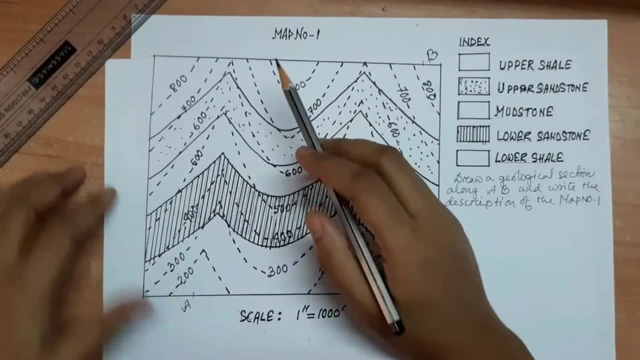 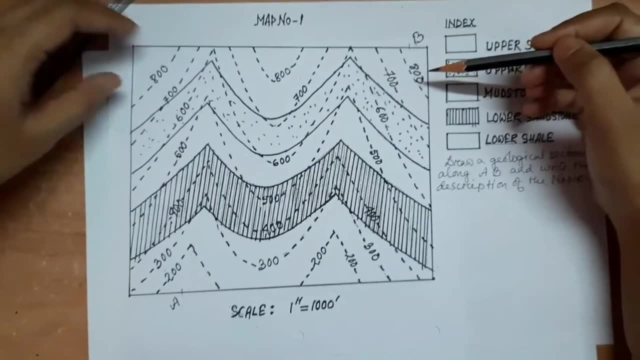 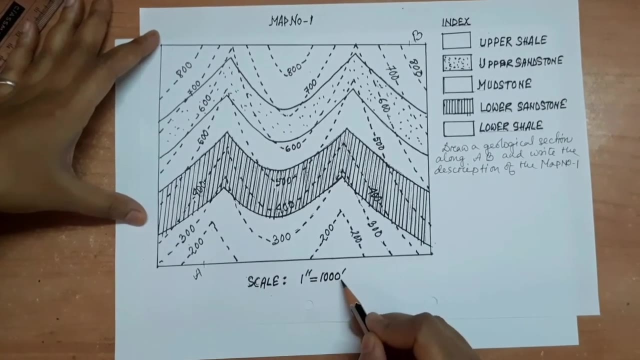 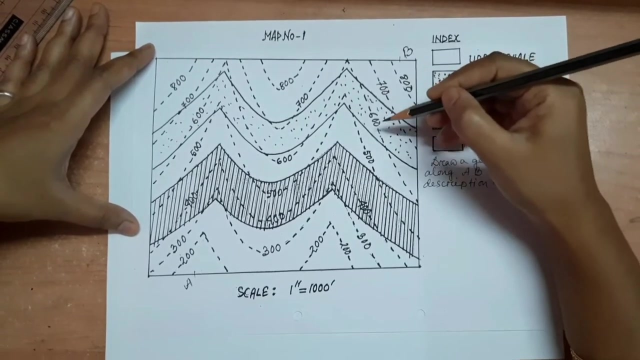 So there are some values. So these dotted lines are known as contour lines And these values indicate elevation. Okay, Now in this map there is a scale. Your scale is 1 inch equal to 1000 feet. So this 800, 800 means 800 feet, 700 feet, 600 feet. Okay, And now come to this continuous lines. 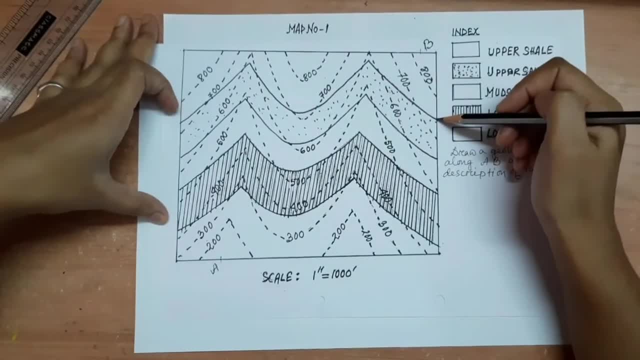 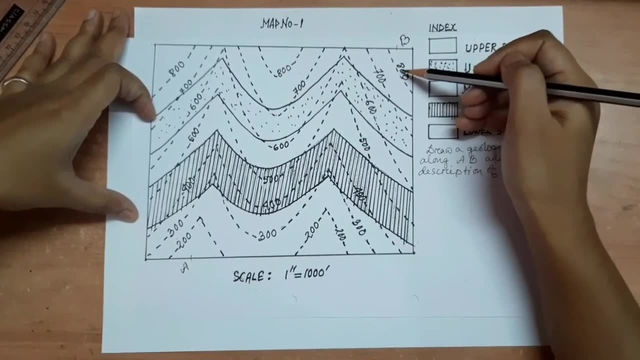 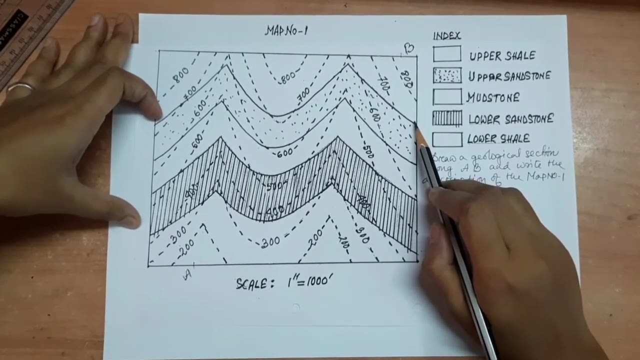 These continuous lines, these continuous lines represent bedding conditions. Okay, These dotted lines are contour lines, These are contour values, Elevation, that means. And these continuous lines, they represent bedding plans. So this is a bedding plan. This is another bedding plan, Again bedding plan. This is again a bedding plan. 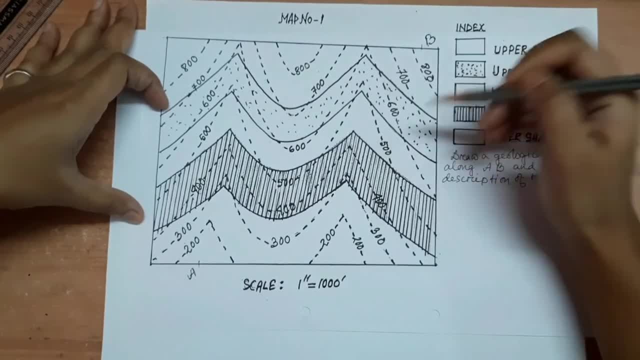 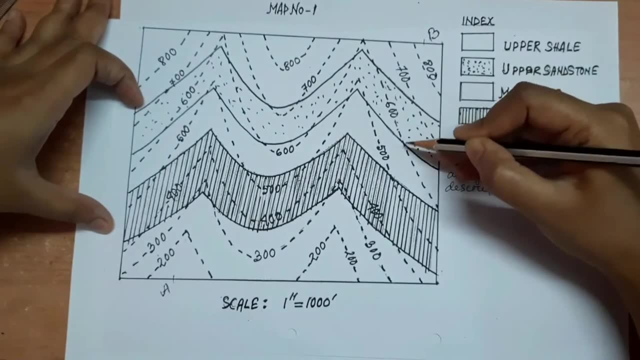 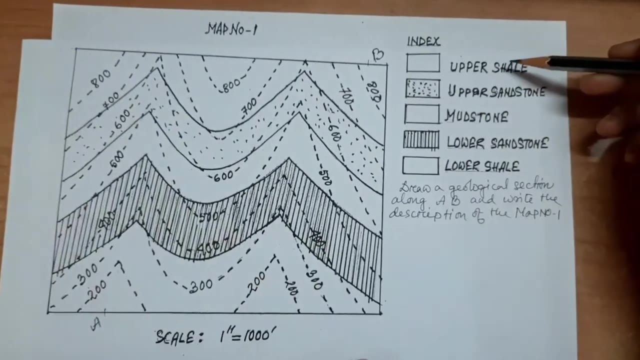 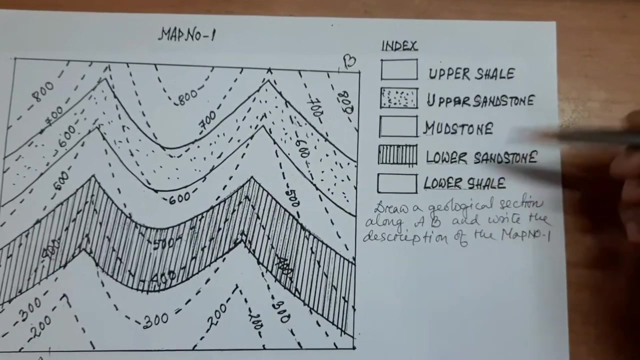 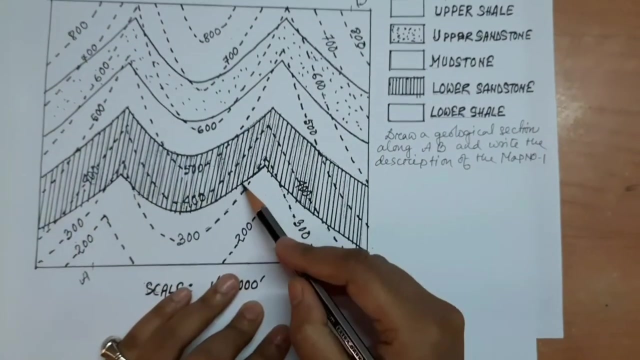 Okay, So these are the bedding plans and the thickness. The thickness between two bedding plans, That means from here to here. This is the point of your bedding plan. Okay, Now, from your bedding plan, another bedding plan is the axis of your bed. that means your. 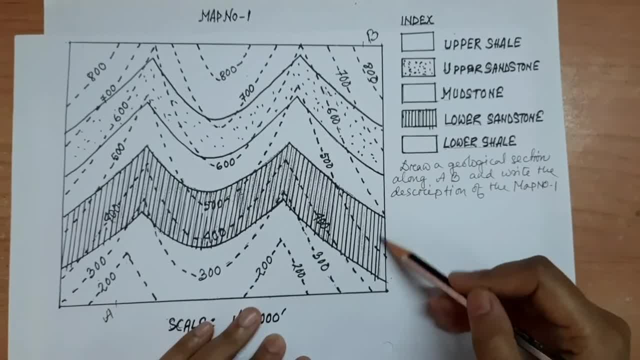 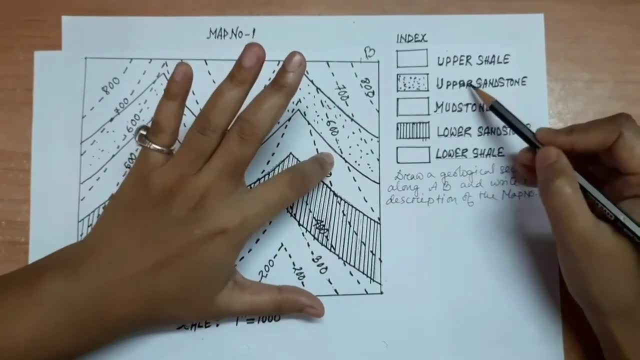 planks. they are faced exactly opposite. Down a net scandals. Okay, They are comingций. So there are a thousand bedding plans here. stone, mudstone bed. this is upper sandstone, this thickness is upper sandstone bed and this is upper. 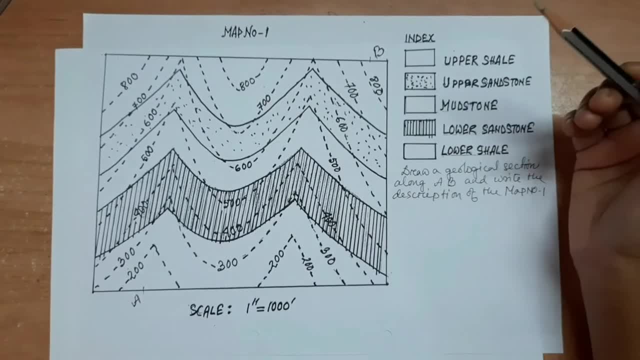 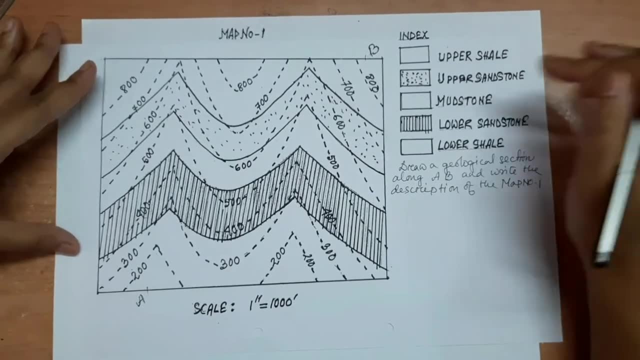 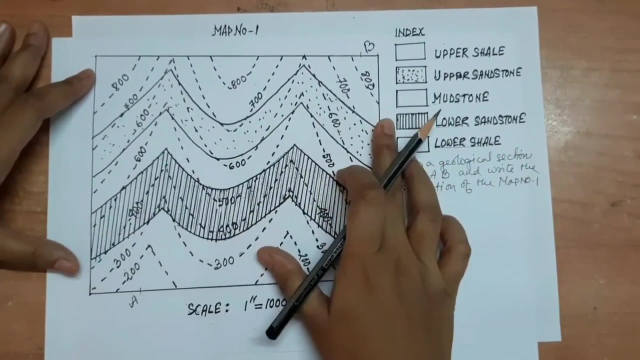 shell. okay, so these are the beds and these continuous lines are the bedding plans. now, to draw a geological section with the help of a geological map, map you have to first you have to draw the strike lines and dip directions. okay, so to draw a strike line first. 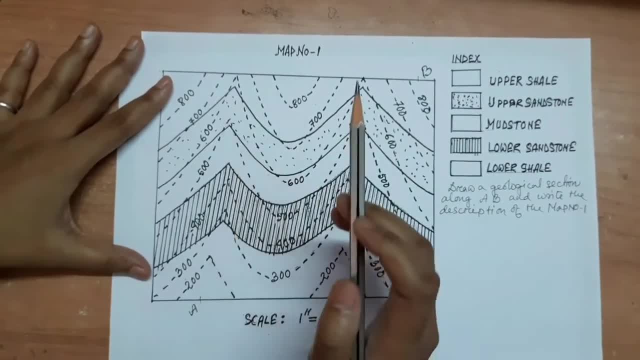 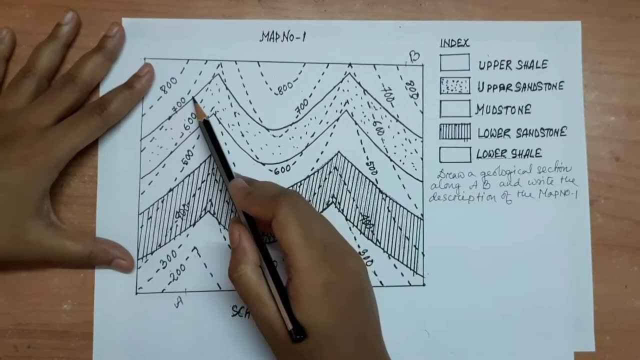 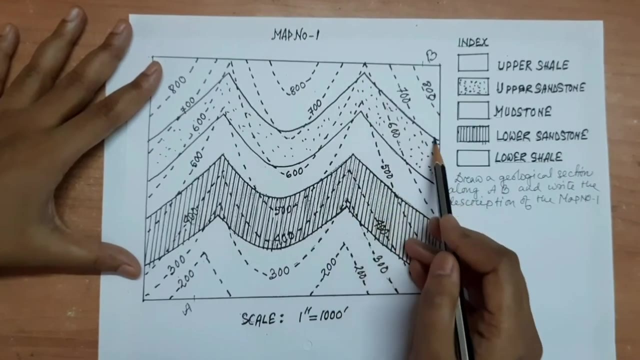 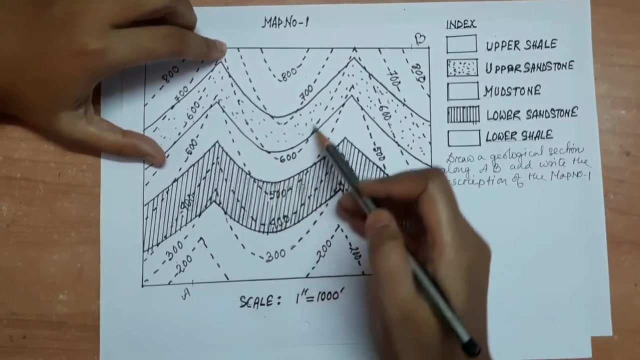 select some intersection points of a contour line, contour line and a bedding plan. suppose this is a bedding plan. okay, this is your first bedding plan and this 600 contour line. this is a 600 contour line and the intersection points are intersection points of 600 contour. 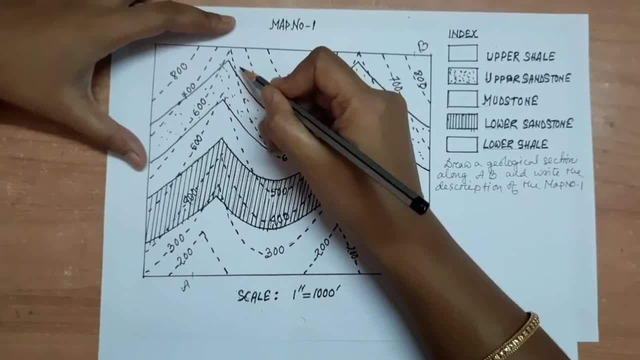 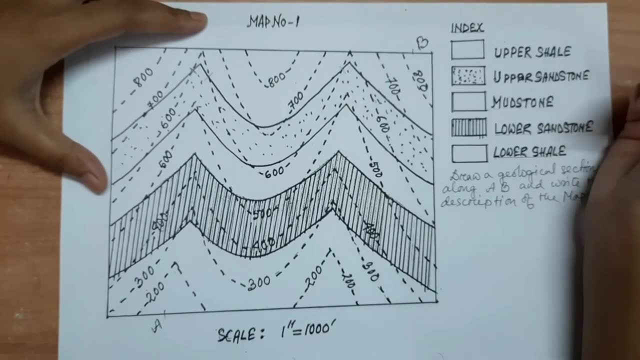 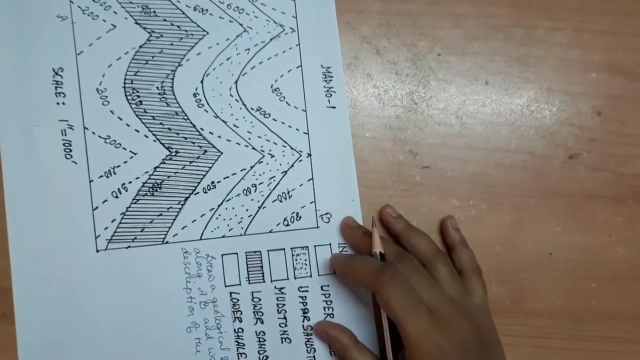 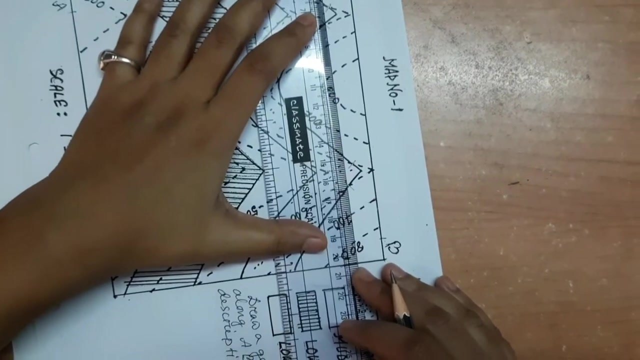 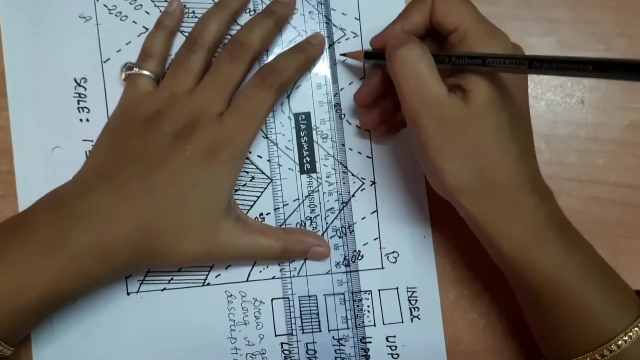 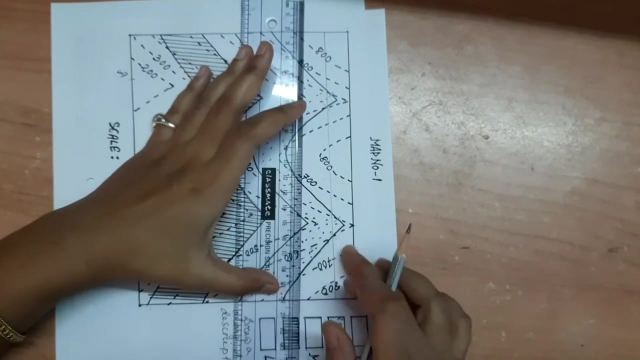 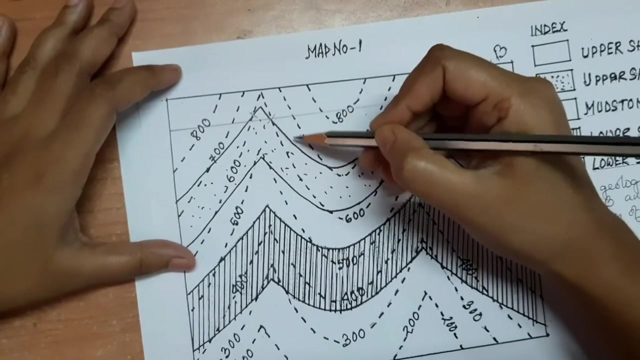 line and this bedding plan is one. is this one? another intersection point, is this one? again, this is a intersection point. this is again another intersection point. okay, so now take any two intersection points, any two intersection points, and join these points. so this is your first strike line. now, this strike line, this bedding plan, intersects the 600 contour. 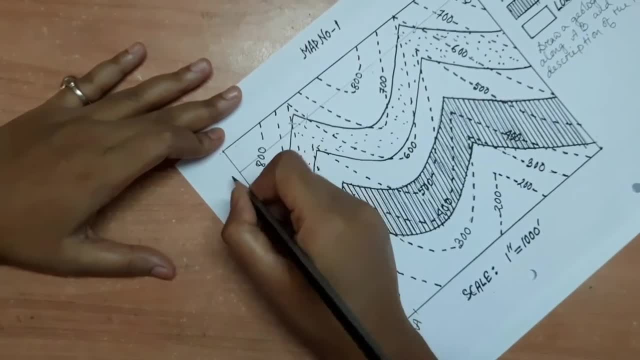 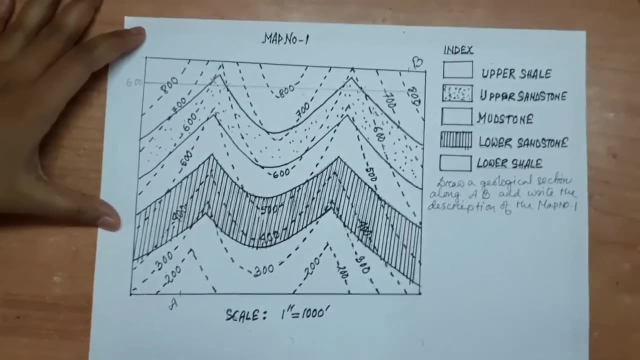 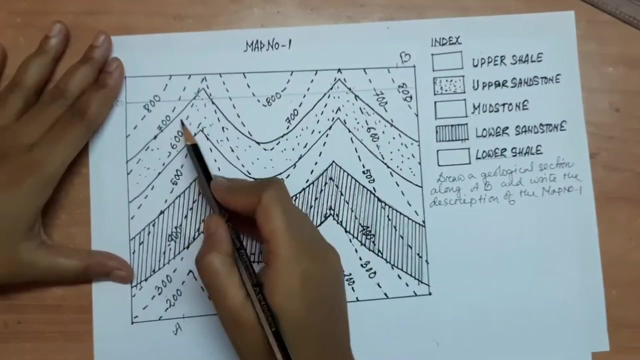 line. so the value of this strike line will be 600- 600. okay, now you have to draw another strike line in the same bedding plan. now you have to take the same bedding plan. you have to find out the same intersection points of the same bedding plan. 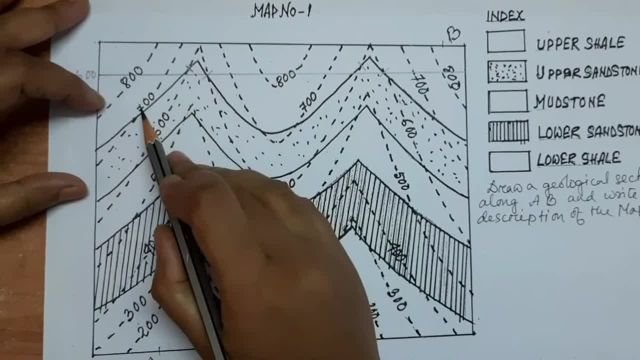 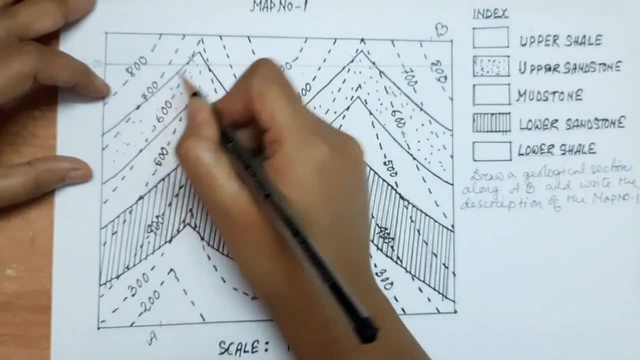 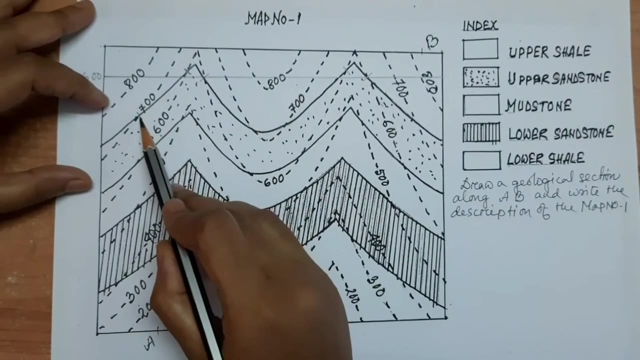 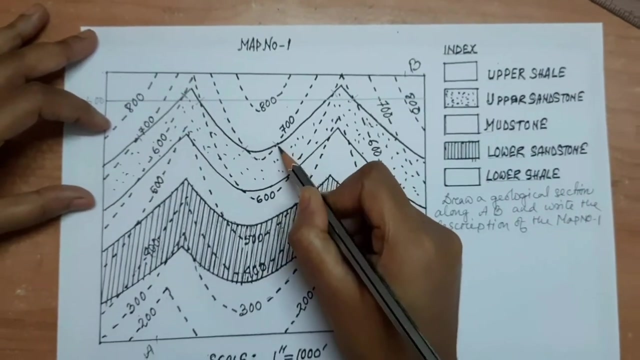 but a different contour line. that means this 700. okay, this is the earlier contour line. was this one 600? now, consider this 700 contour line and the same bedding plan. okay, so this is a intersection point here. this one is another intersection point. this one then. this is a intersection point. 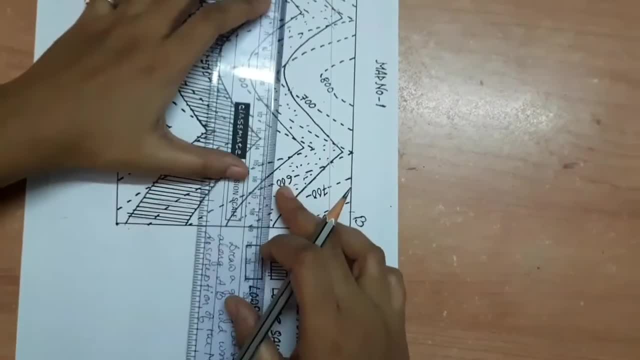 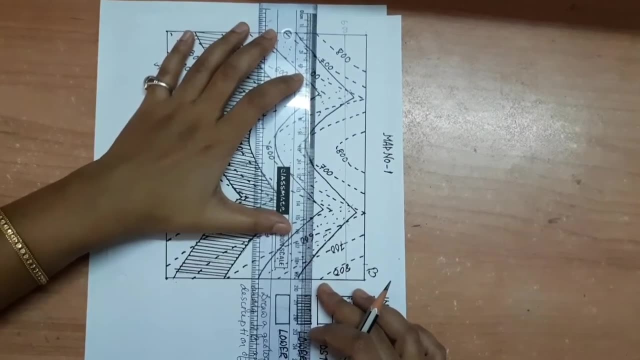 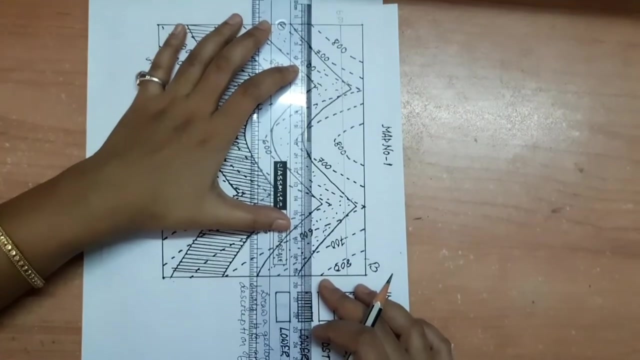 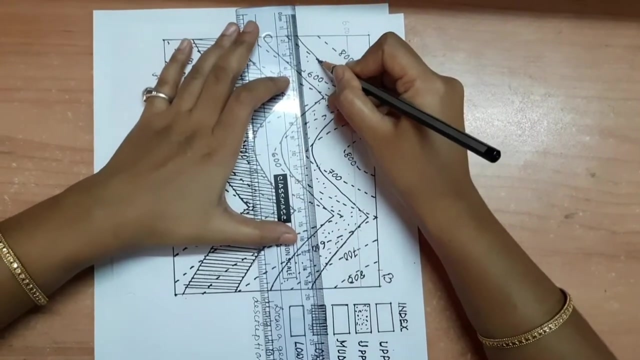 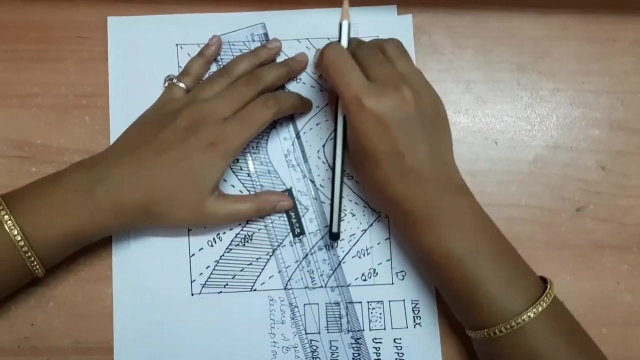 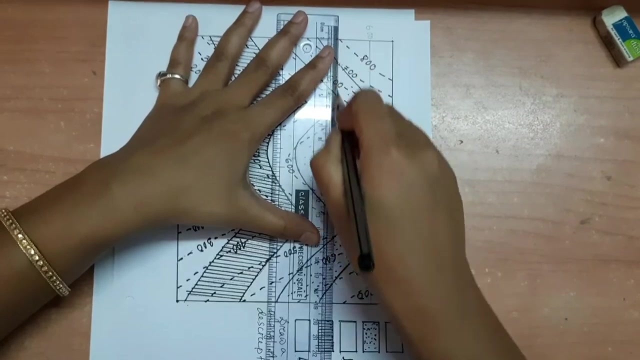 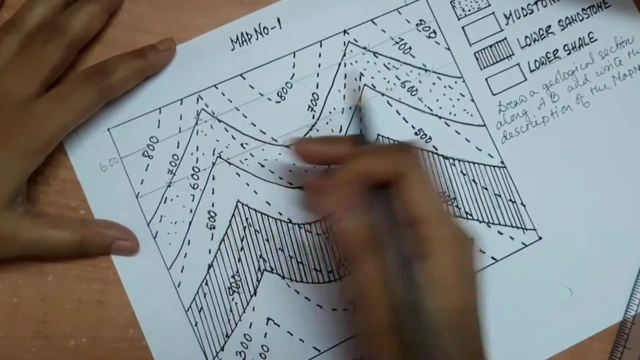 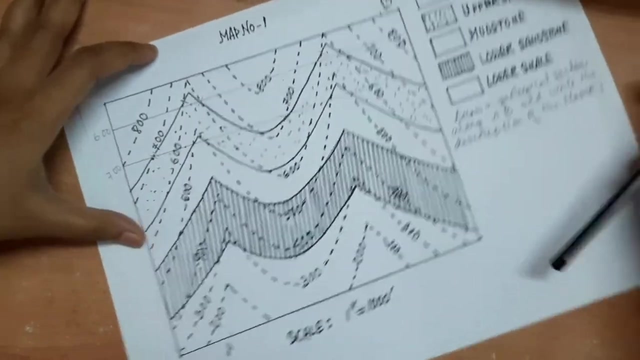 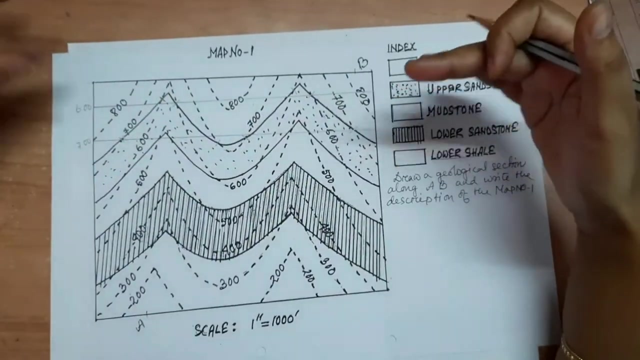 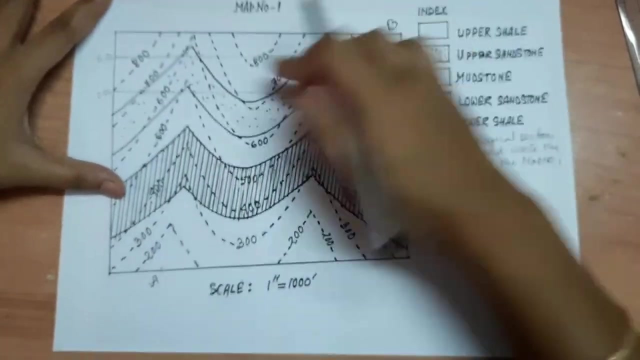 now again, join these points. you can join any two points. this is your intersection point, so so join this point. so we take a referencing point, which is: dogs is, this is your rock bed, this is your bedding plan and this is the trend, okay. strike line indicates the 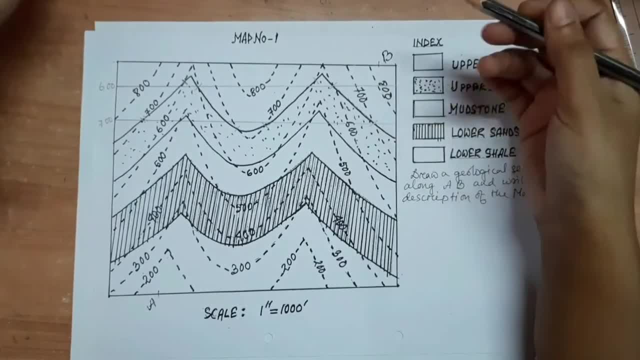 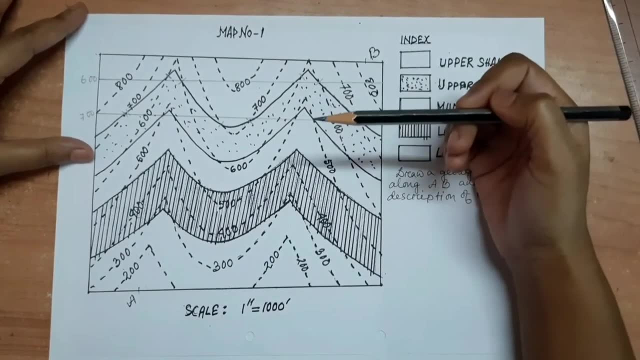 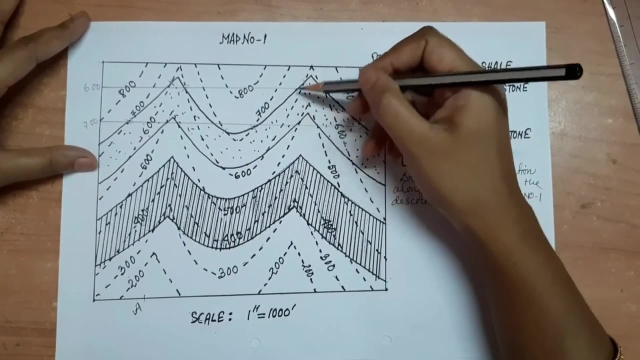 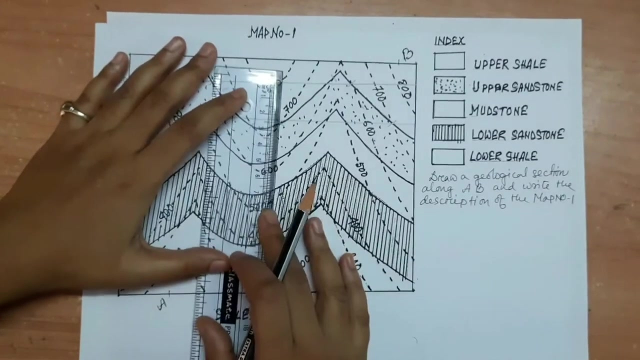 trend of the rock mass or strike line is what strike line is? a intersection line between the bedding plan and then imaginary horizontal plane? okay, so, and we know that two strike lines are always parallel. so it must be parallel, this strike line and this this. it must be parallel, okay. 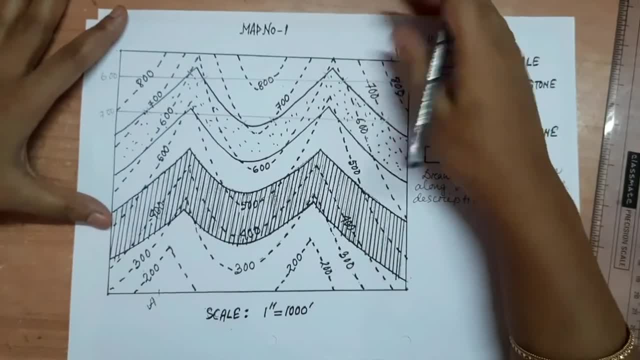 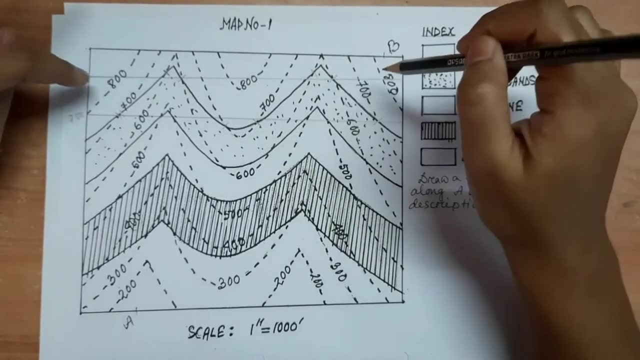 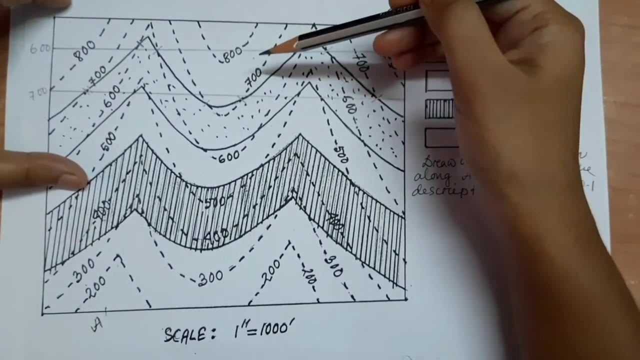 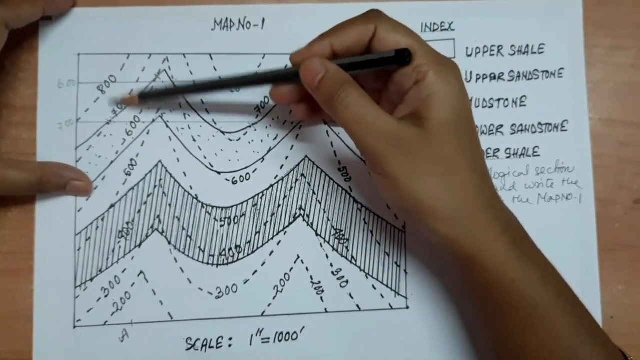 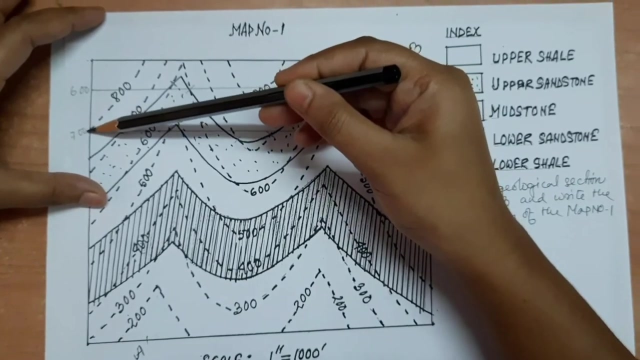 now. now, what is the deep strike line is the intersection line between the, between a bedding plan and then imaginary horizontal plane, and deep is the deep is the inclination of the bedding plan. that means deep is the vertical drop. now, here you can see, these are two bedding plans. value of this bedding plan is 700 feet. this is 600 feet, so 700 minus 600. 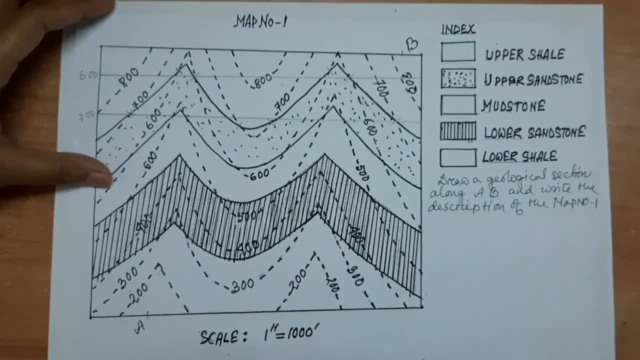 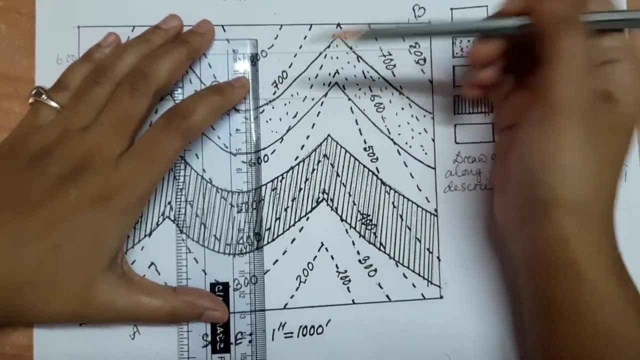 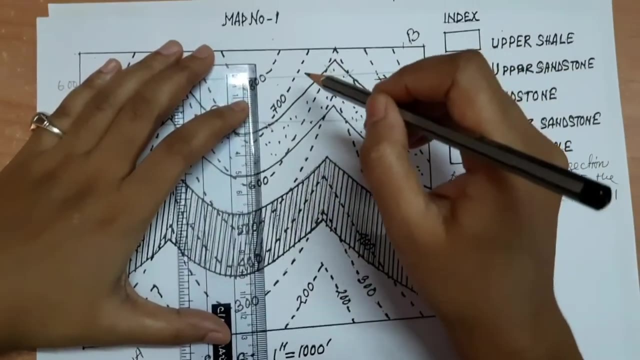 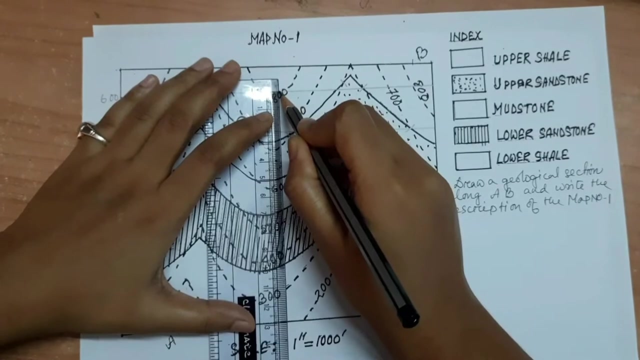 your vertical drop is 100 feet, 100 feet. so draw a perpendicular line. perpendicular line why? because we know that strike lines and deep and deep and the strike line, strike and deep is all. I was perpendicular to each other. so draw a perpendicular line. now, your vertical drop is: 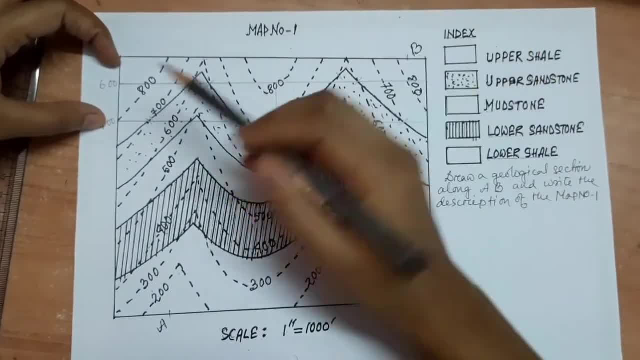 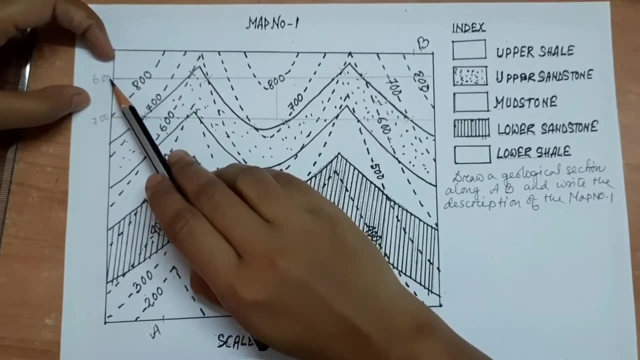 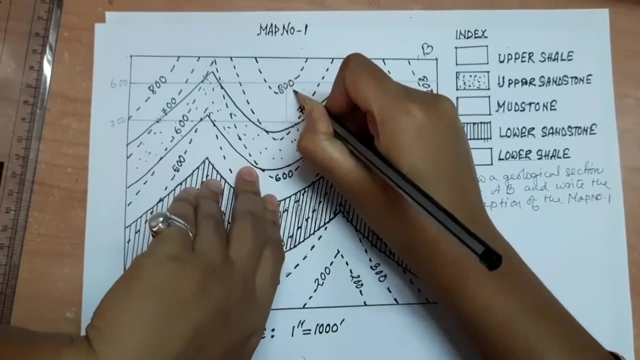 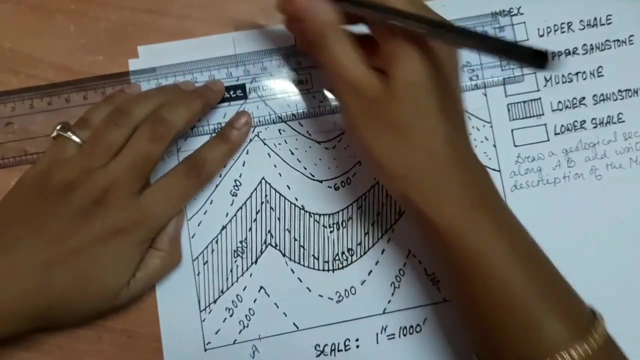 100 feet, hundred feet towards which direction? this is seven hundred higher elevation, then, and this is 600, that means lower elevation, that means your inclination is towards this direction. okay, so this is your deep direction, okay, so so, If this is north, south, east and west, 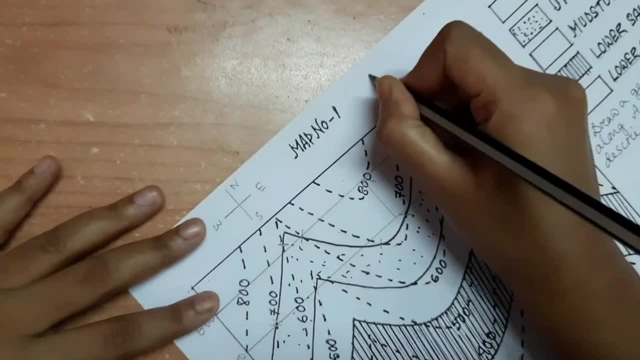 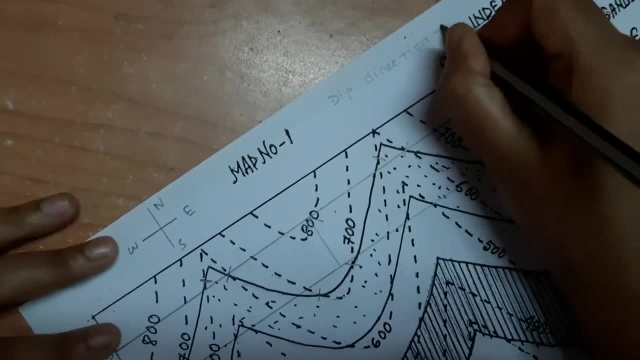 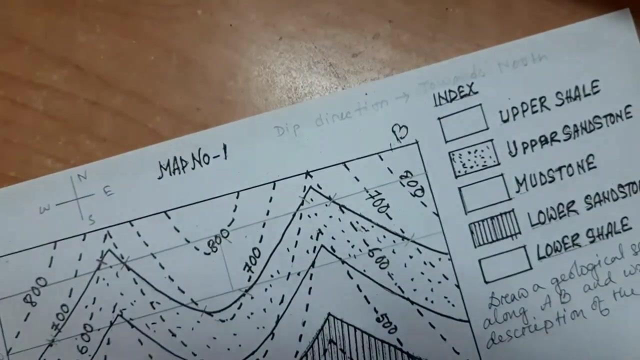 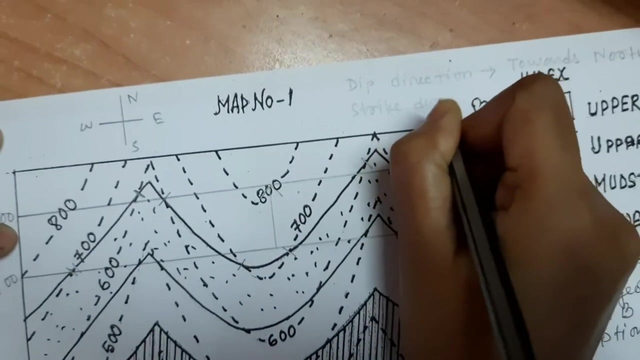 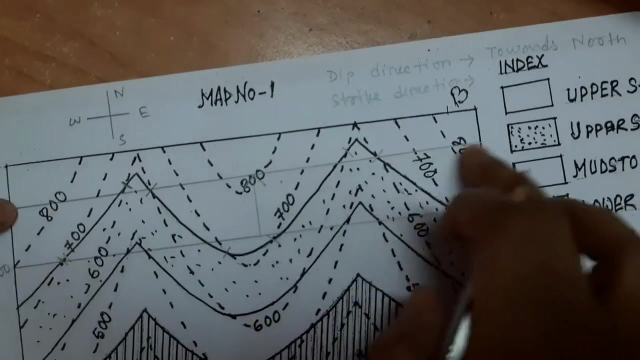 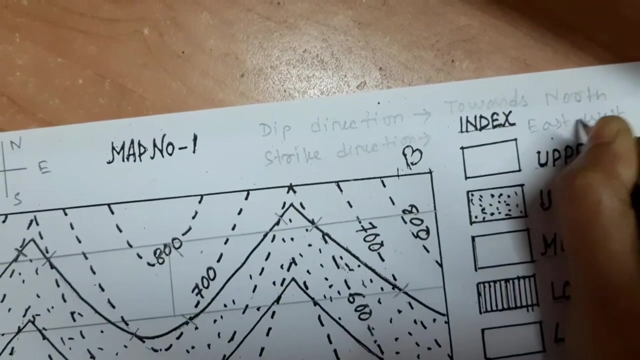 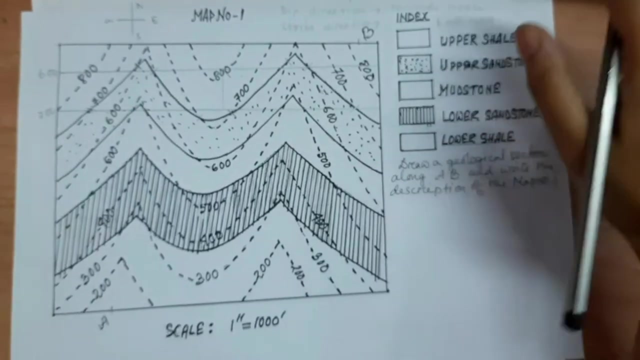 So your dip direction is towards north. Dip direction, Dip direction is towards north. Okay, Now what is your strike direction? Strike direction is: Strike direction is east to east. Okay, this is the strike direction. So strike direction will be east to east. So these are all about dip direction and strike direction. 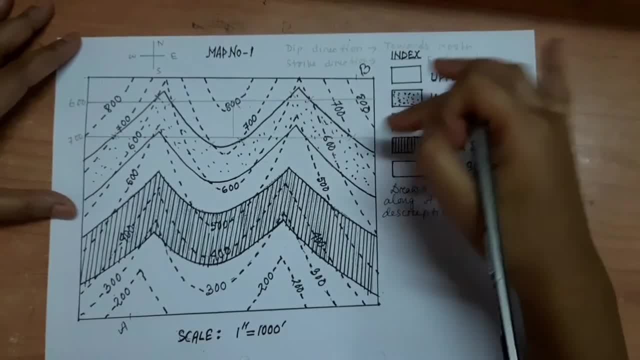 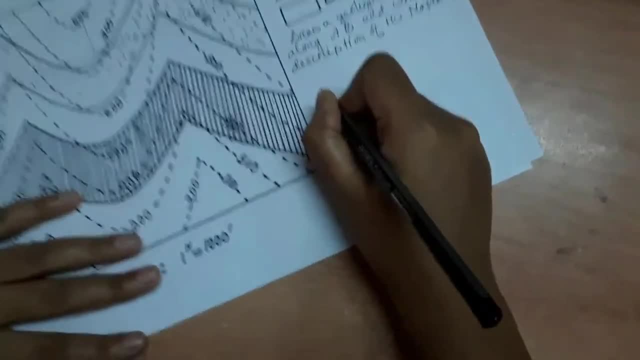 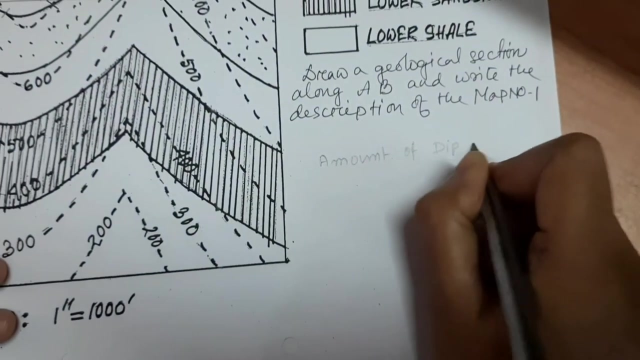 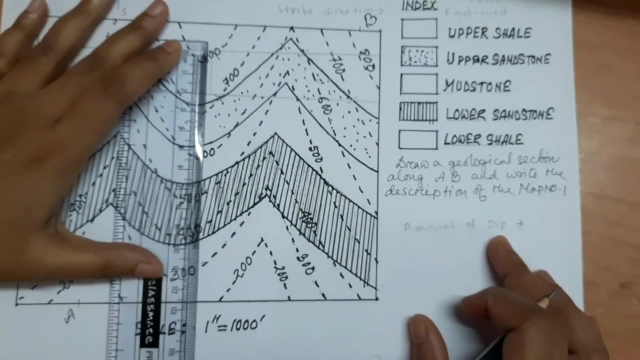 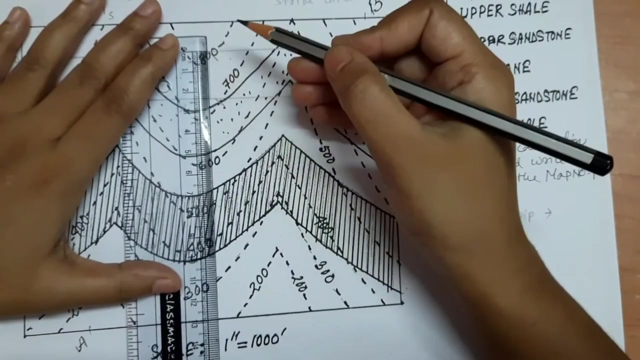 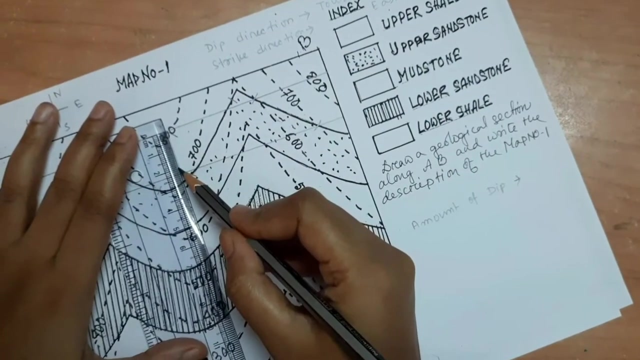 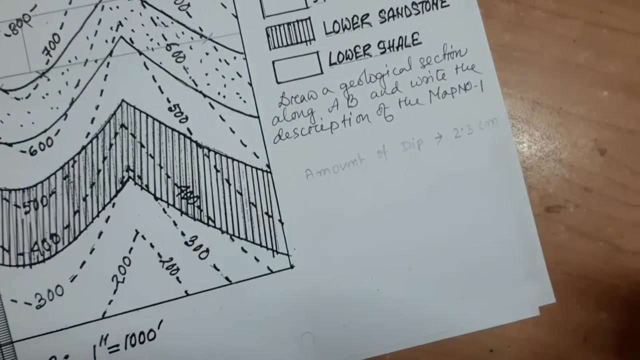 How to draw dip and south Strike in a geological map. Now, How to draw a dip amount, Amount of dip. So to draw the amount of dip or dip angle, First measure this line, This perpendicular line. This is 2 point 2.3, 2.3. 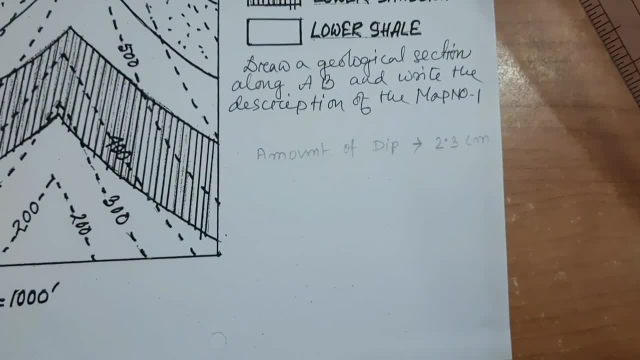 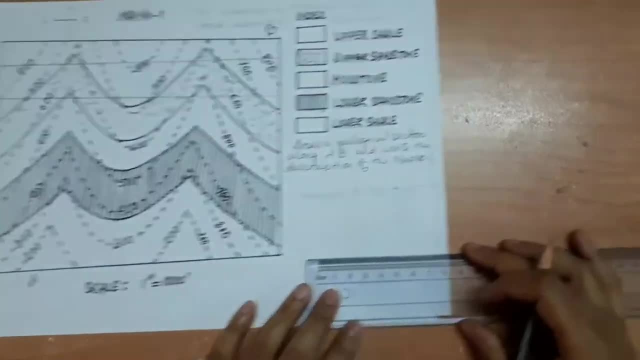 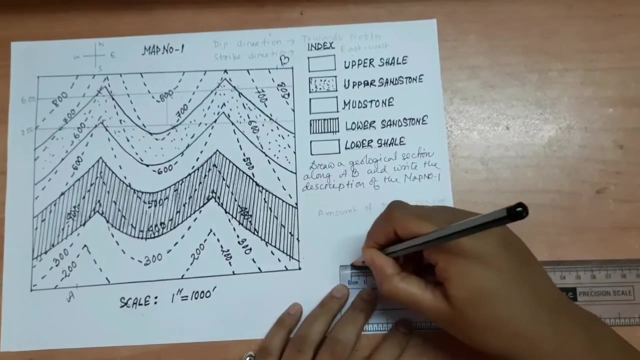 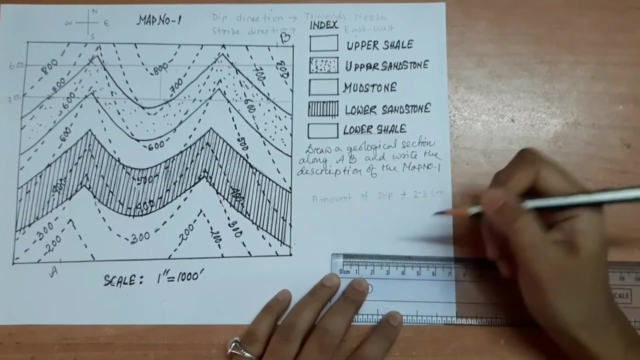 Now here Come to the scale. Scale is 1 inch equal to 1000 feet. Okay, So Draw this, Transfer this to the scale. So for this perpendicular line, 2.3. This is 2.3, Now, 1 inch equal to 1000feet. 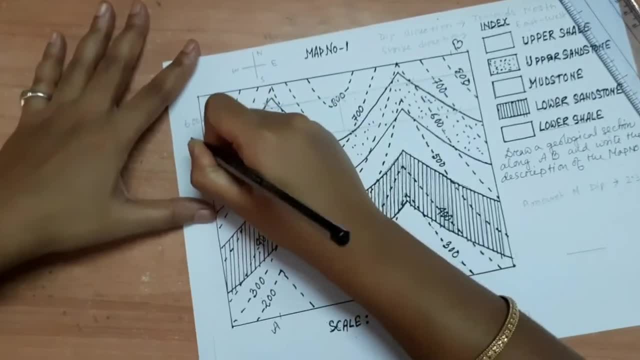 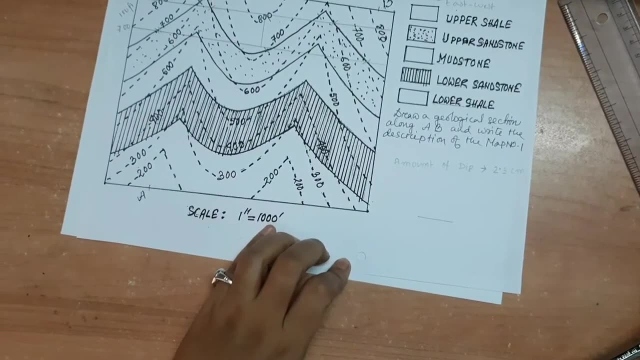 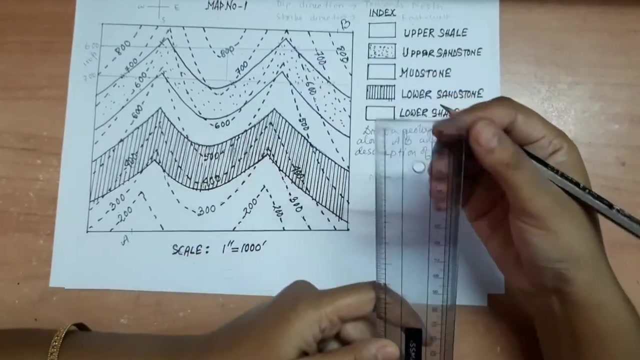 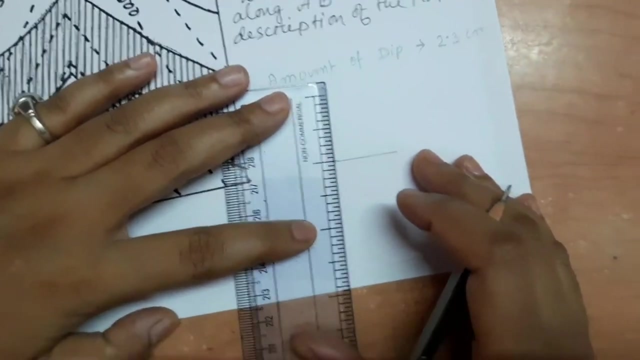 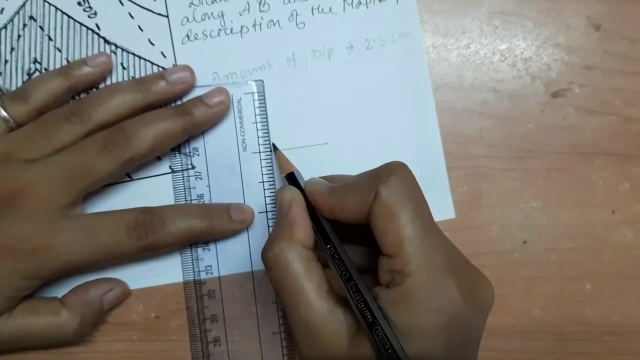 So Your vertical drop is 100 feet, Vertical drop is 100 feet. So If 1 inch equal to 1000 feet, Then 100 feet will be 100 feet will be 0.1 inch. Okay So 0.1 inch means 0.1 inch will be somewhere here. Okay So, 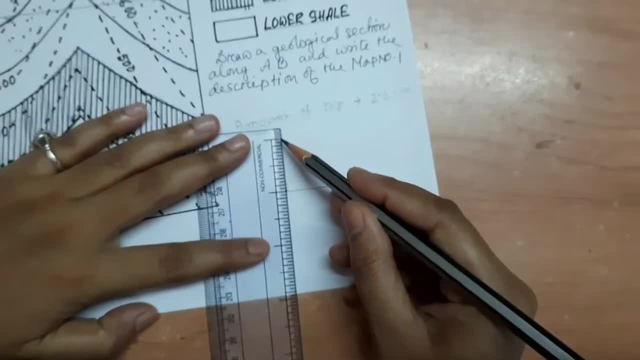 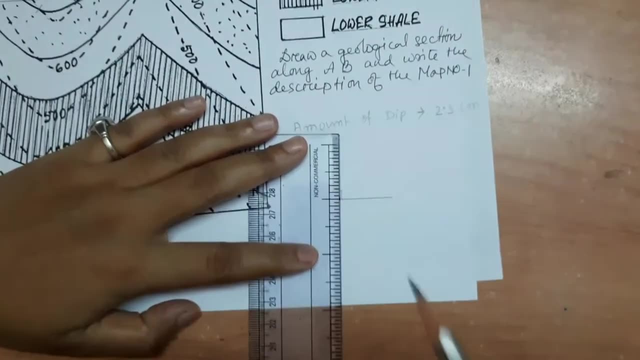 in this scale- I am using this scale here- There are eight divisions. One inch equal to 1,, 2,, 3,, 4,, 5,, 6,, 7, 8 divisions. Okay, That is why in this scale, 0.1 inch will be. 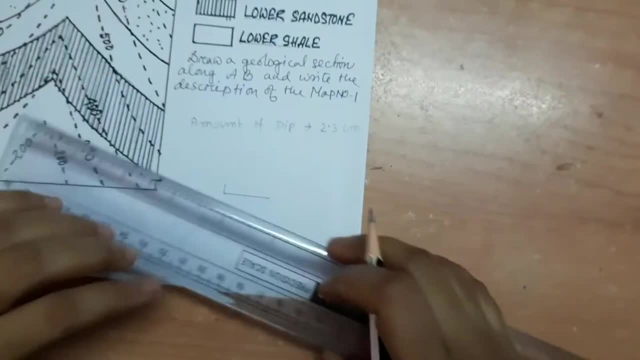 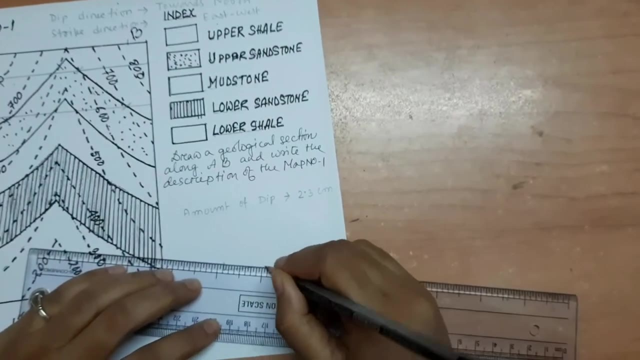 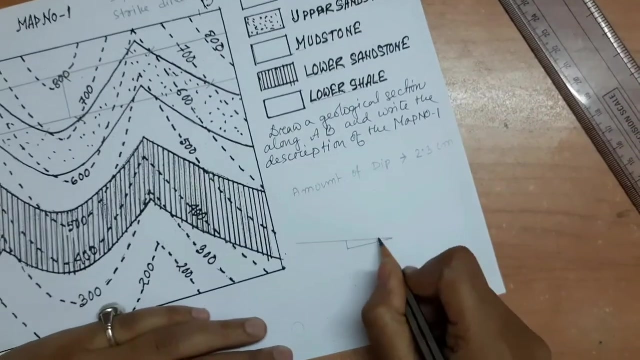 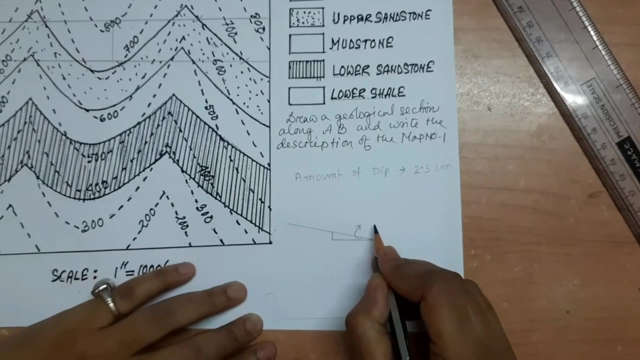 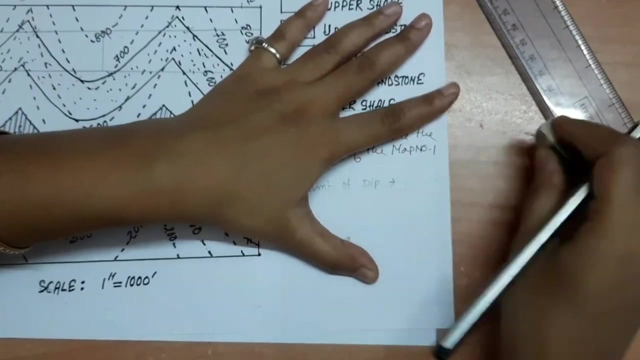 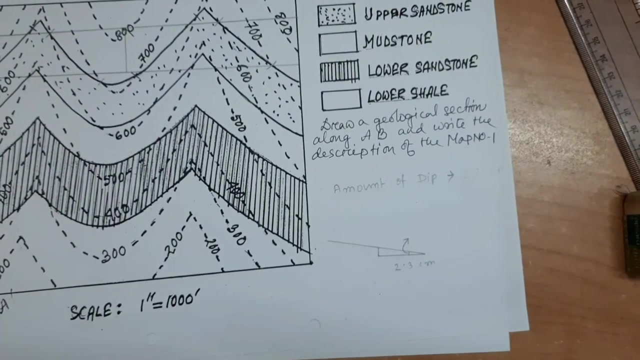 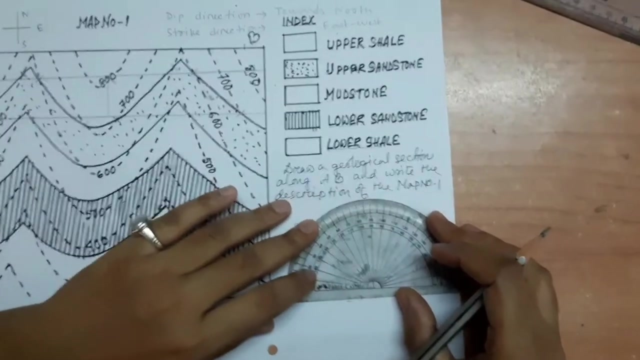 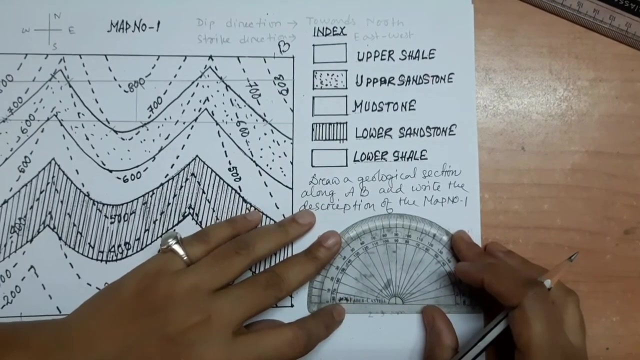 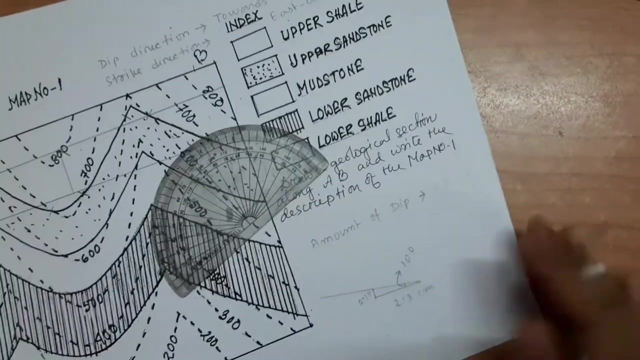 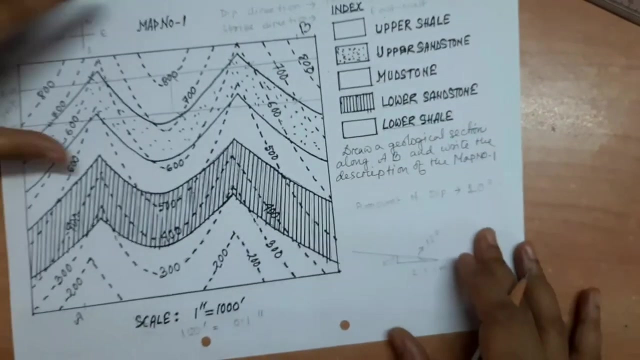 somewhere here. Okay, Now join these two points. Now measure this angle, This angle, and this will be your deep angle or amount of deep. Okay, This is 2.3 centimeter. Now measure this angle. So this is a 10 degree angle. So your amount of deep will be 10 degree. Okay, So strike. 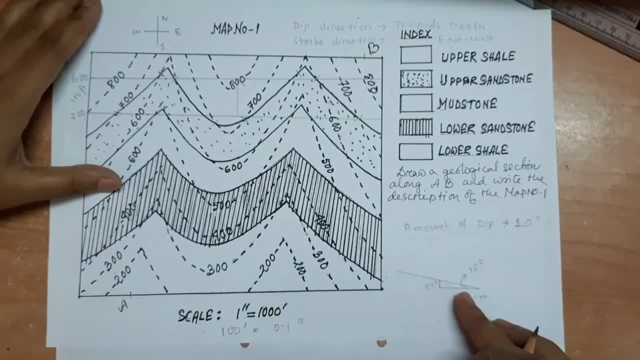 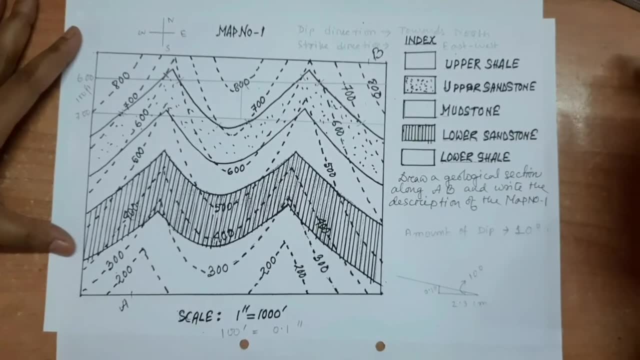 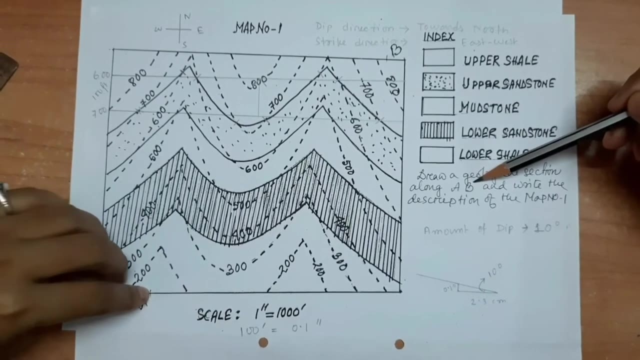 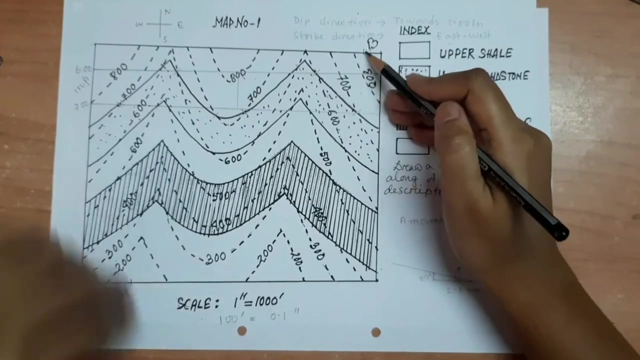 direction, deep direction and amount of deep. Now to draw a geological section in here- this is your question- And draw a geological section along AB. That means this is a point here, This point is A and this point is B. Okay, Along this line you have to draw the geological section. So 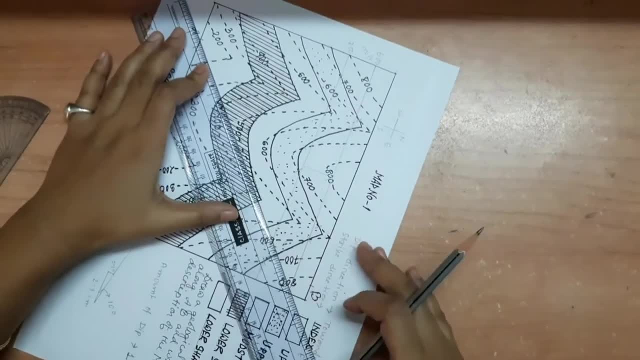 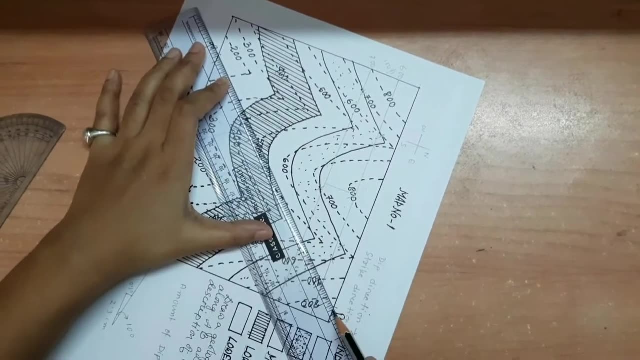 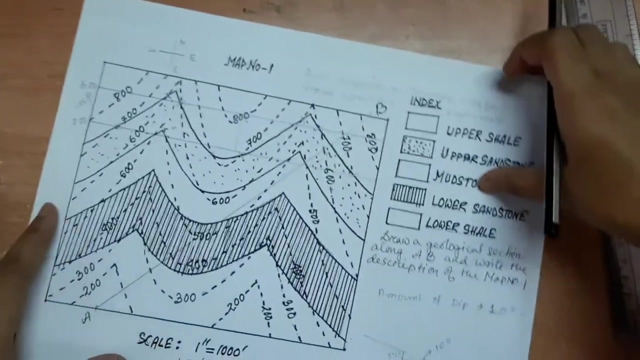 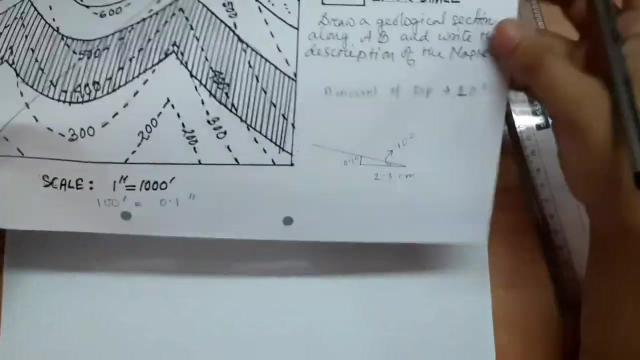 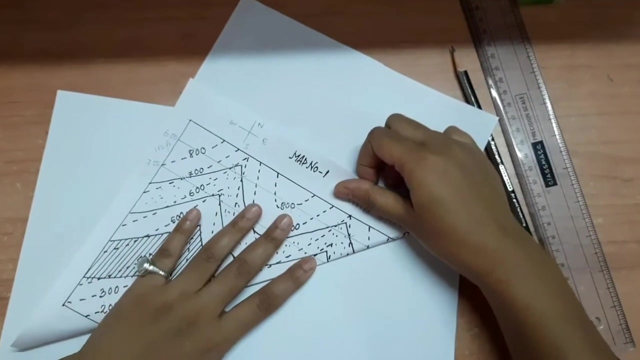 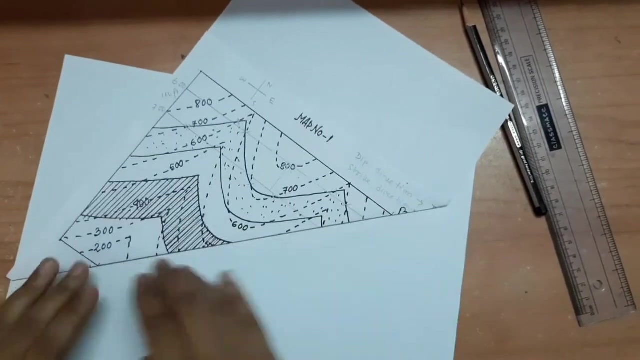 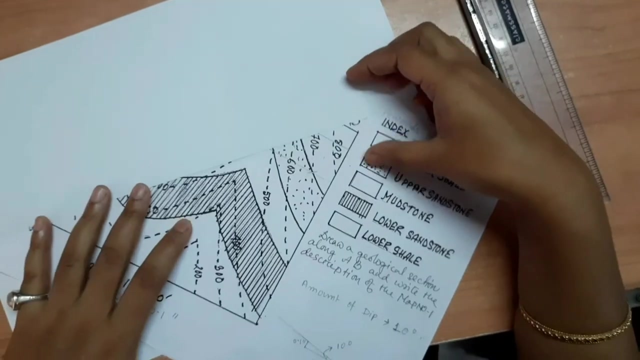 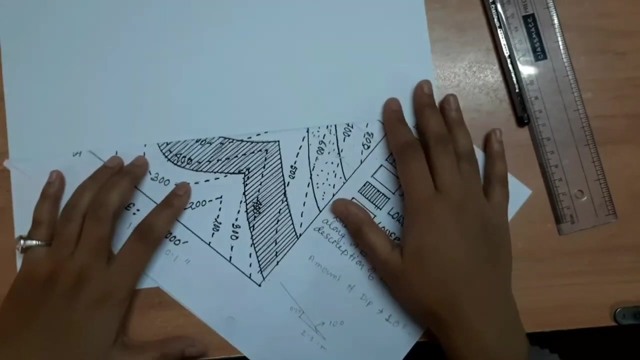 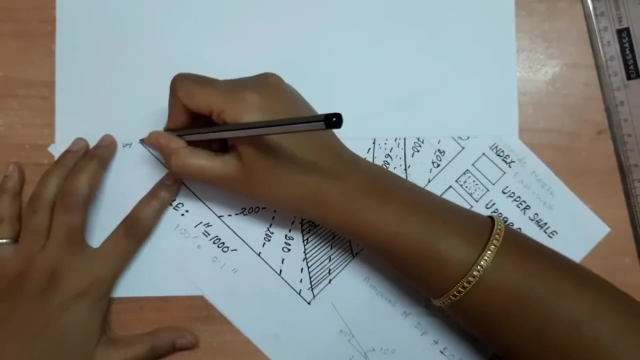 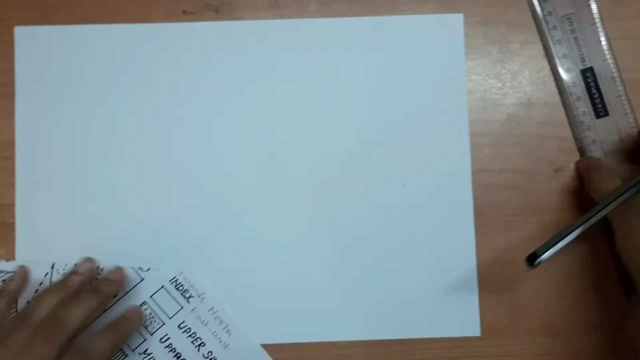 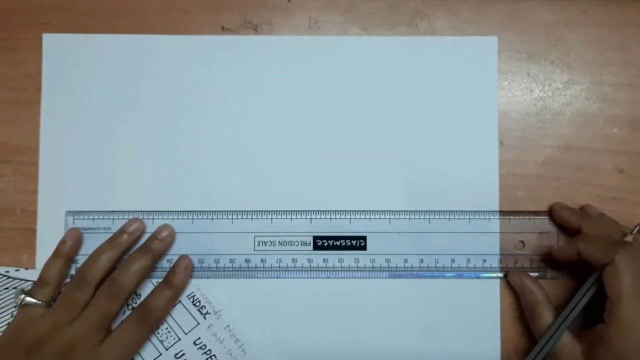 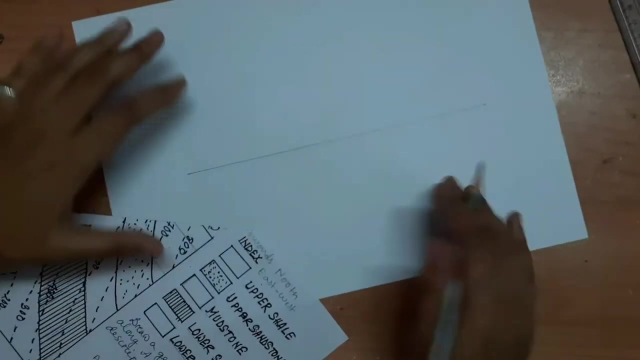 first join these points A and B: A and B. Now fold this paper along AB. Now fold this paper along AB. Now, this is it. This is point A, point A and this is point B. Okay, This is A and B. 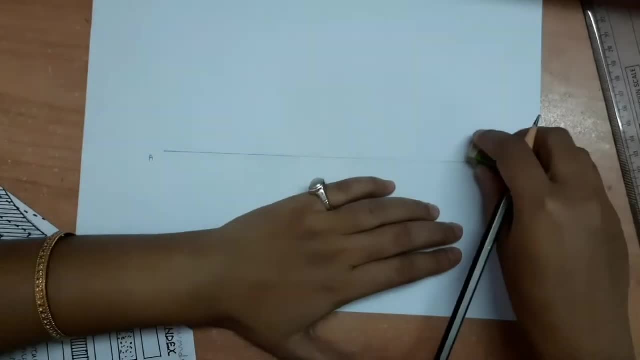 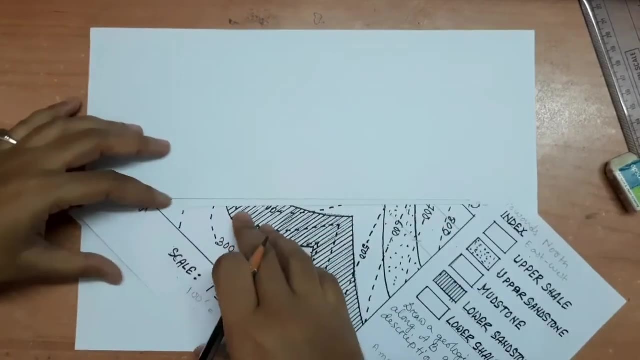 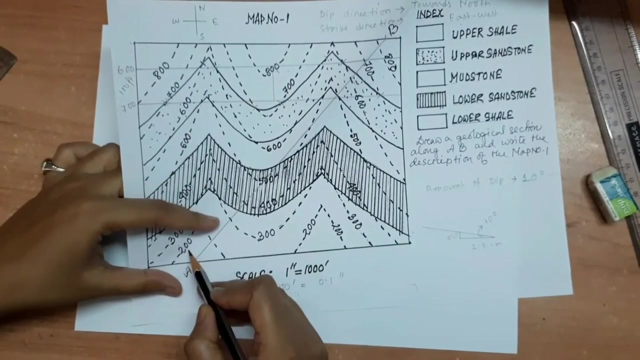 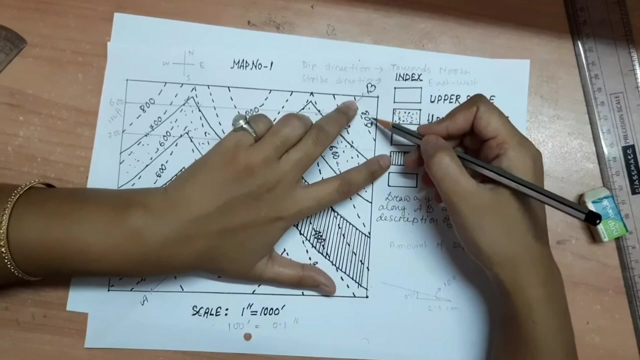 Now, now value of A is. value of A is less than 200.. Okay, Less than 200,, but more than 100.. Okay, 100 feet, And here value of 800 is, uh, greater than 800.. 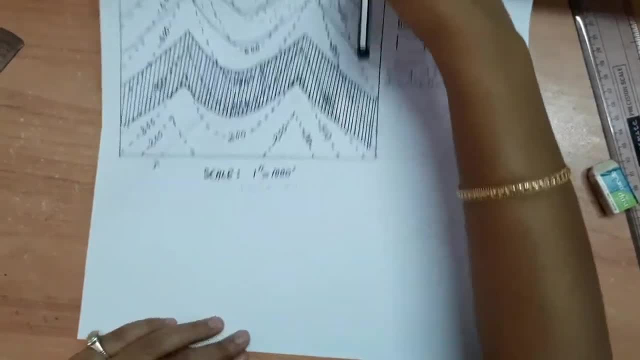 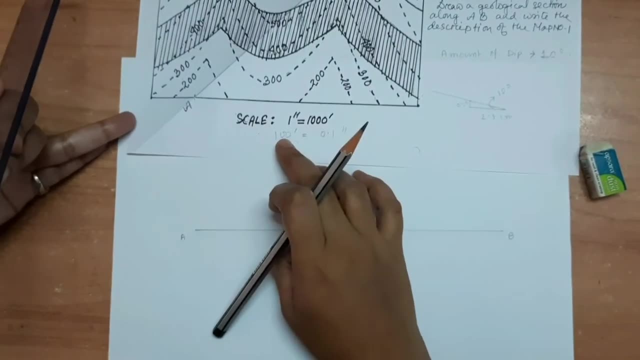 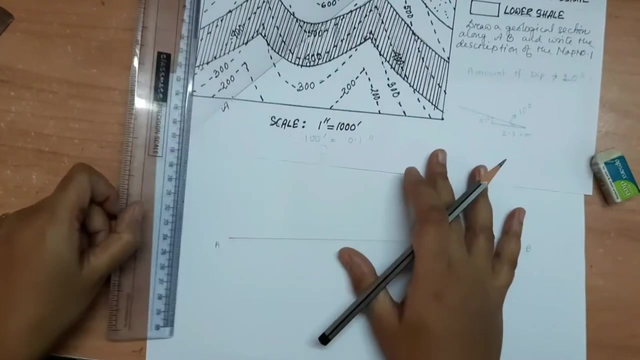 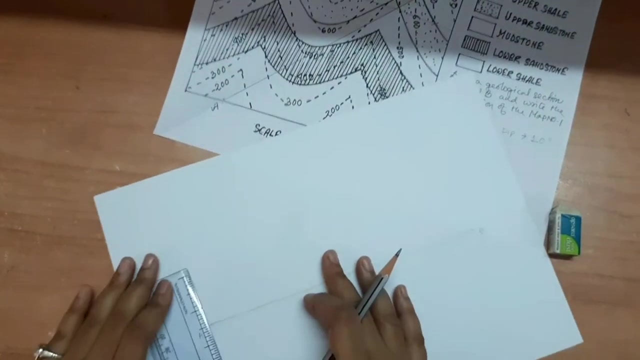 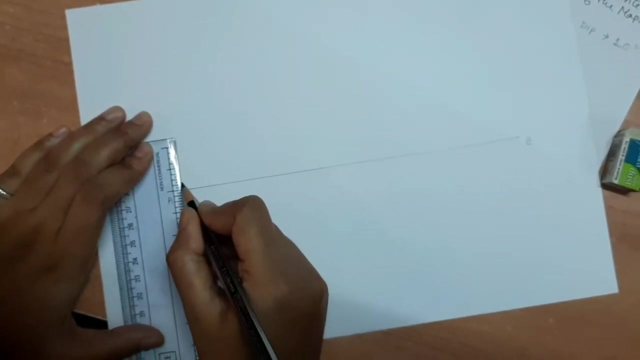 Okay, So 800 means 800 feet. Okay, Now we know that 100 feet equal to, uh, 0.1 inch equal to 100 feet, Then 800 feet will be. This is 0.1 inch. 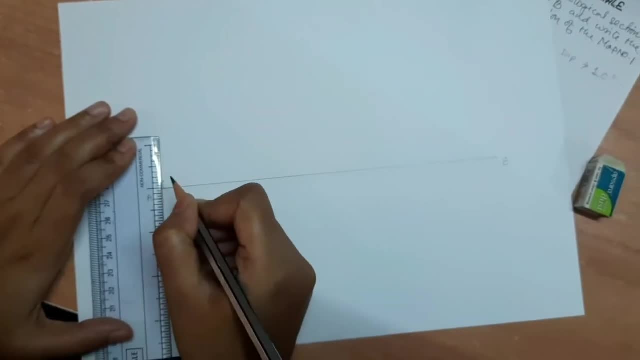 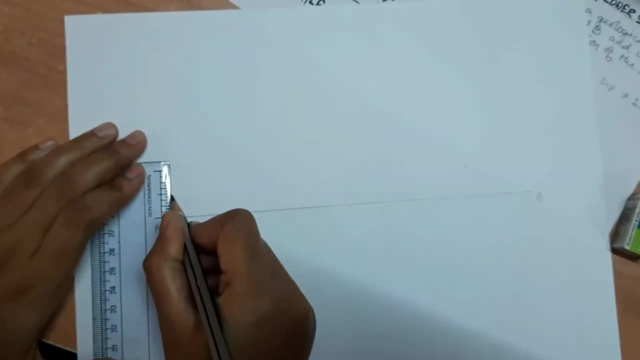 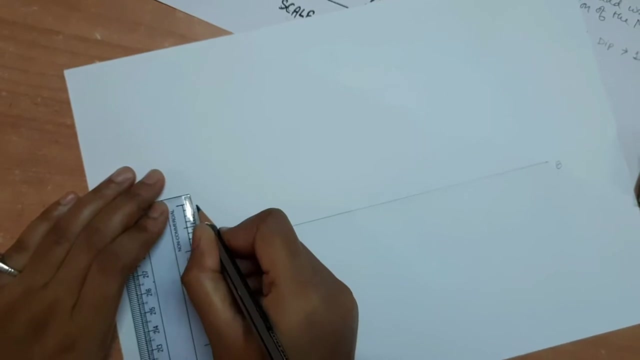 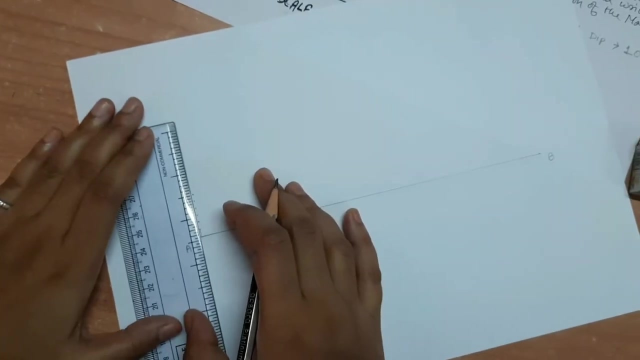 Okay, 0.1 inch. Then Again, this is 0.1 inch: 100, 200.. Then this is 300. 400., 500. 500.. Then 600. 600. 700.. 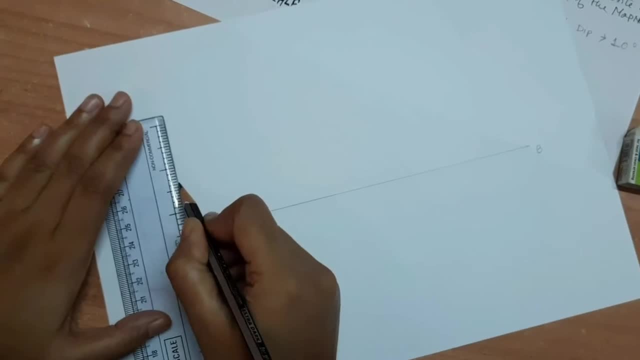 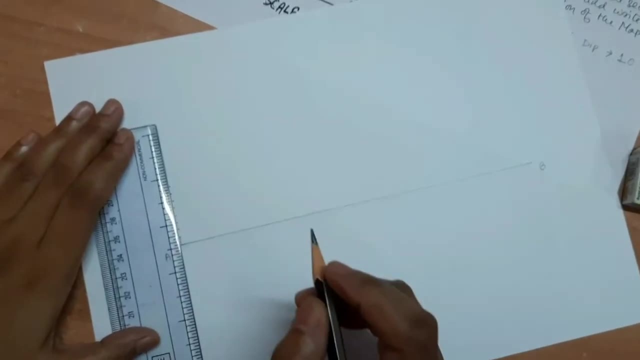 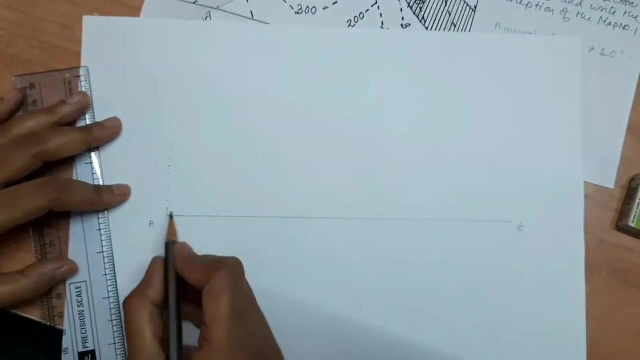 500.. 800.. 100, 1.. This point A is okay. Okay, But Because you know, there are these points which, what I would call the point, is private, starting from zero to close. Let's say it wouldn't be 400.. 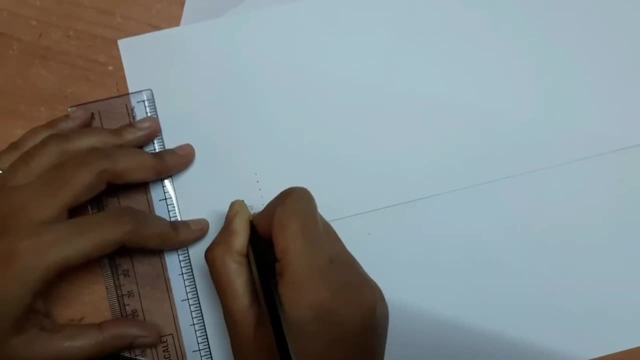 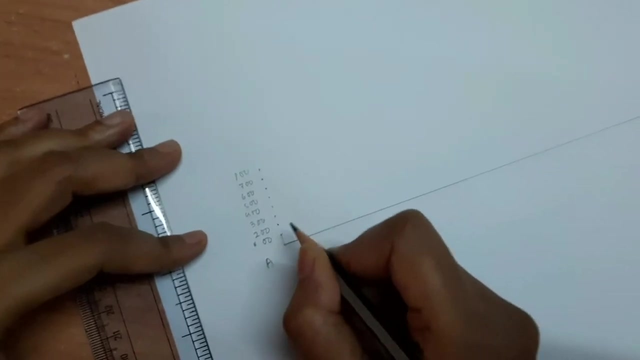 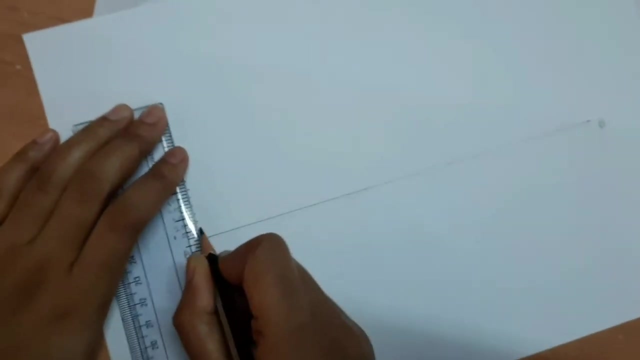 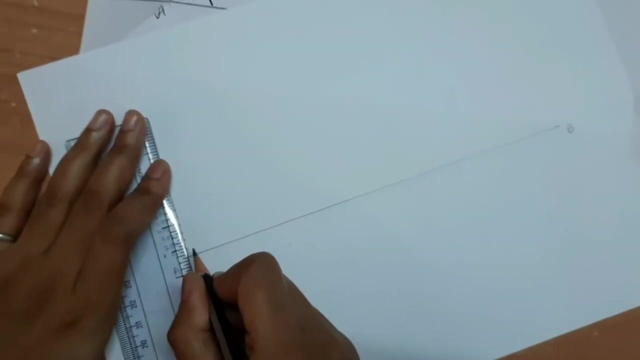 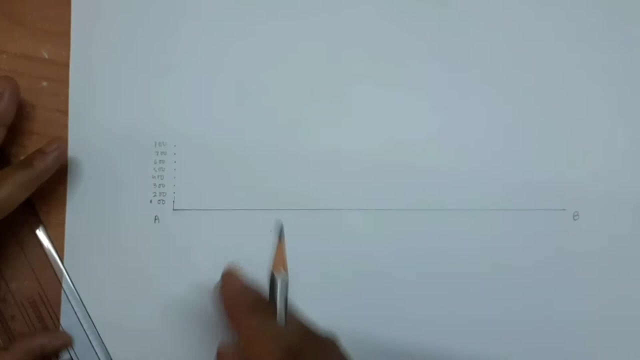 Do not understand 300, 400.. So point A will be this one: 200, okay, Less than 200, that means somewhere in between this 200 and 100.. Suppose this point, this point Now B, is more than greater. 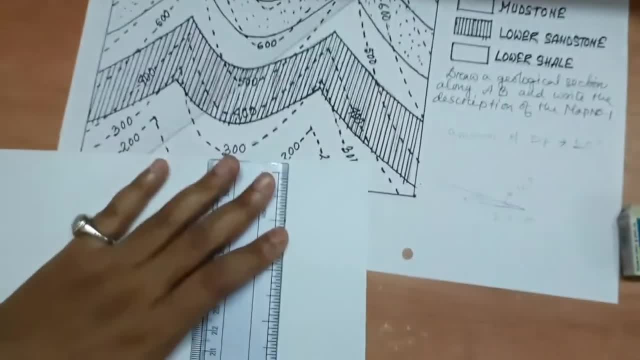 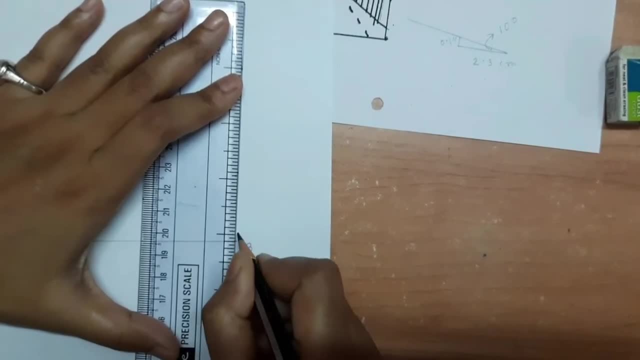 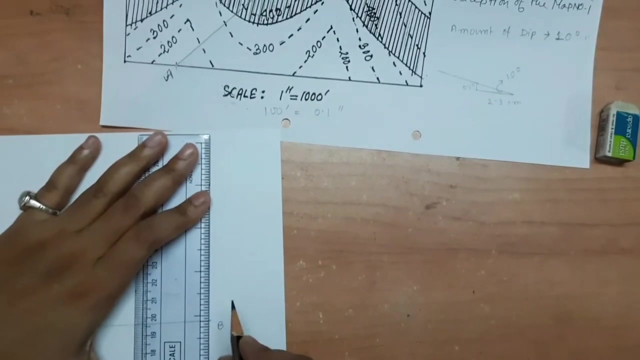 than 800, okay. So if 1 inch equal to 0.1 inch is equal to here, 0.1 inch equal to 100 feet, So 800 feet will be 0.8 inch. okay, More than 0.8. 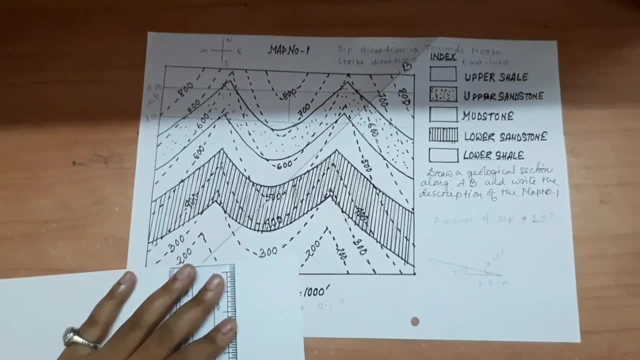 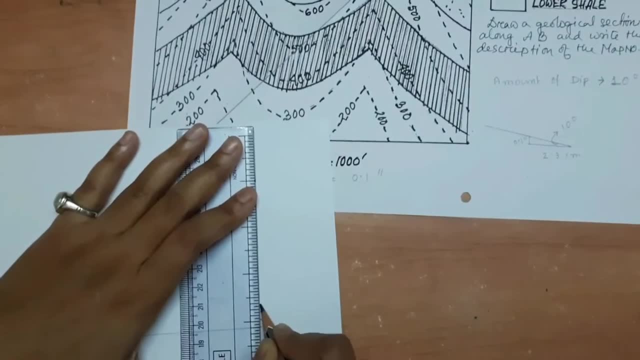 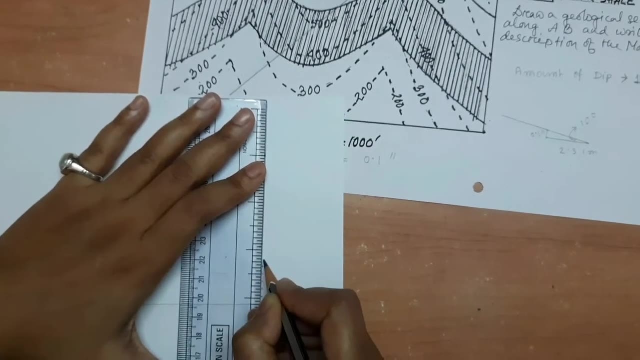 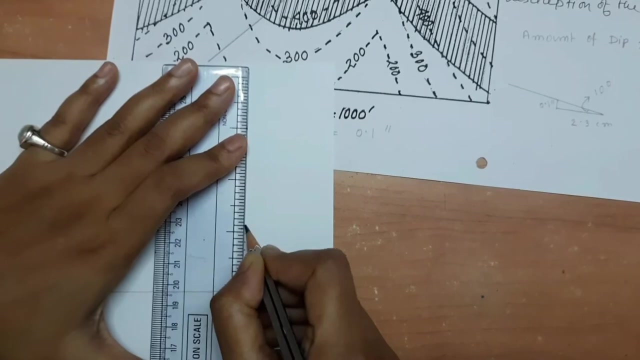 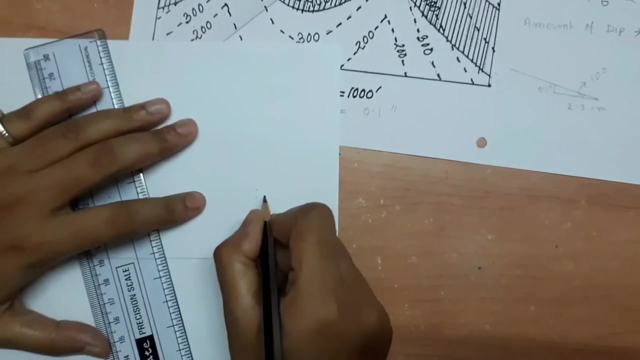 inch, because it is more than 800,. okay, So this is 0.1, 0.2, 0.3, 0.4, 0.5, 0.6, 0.7, 0.8, 0.9.. So B is in between 800 and 900,, 800 and 900. So it will be somewhere here. 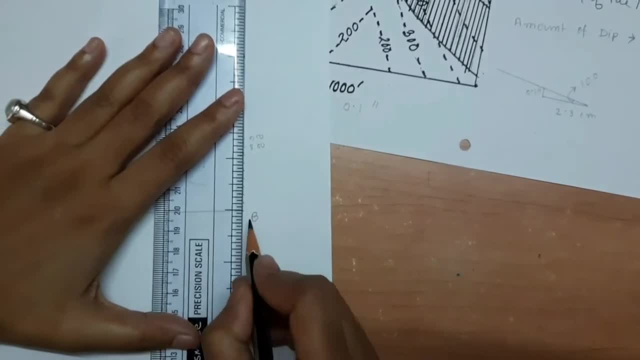 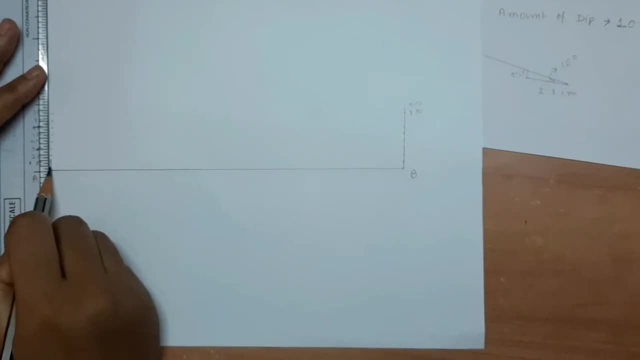 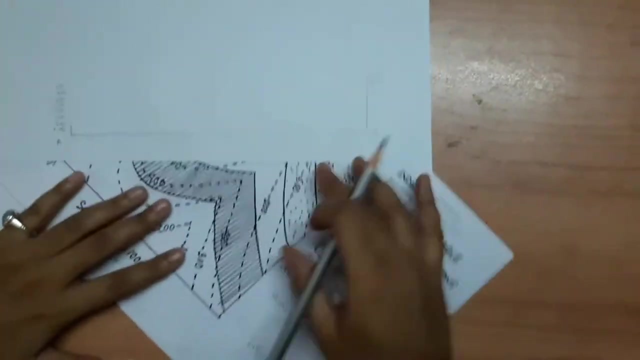 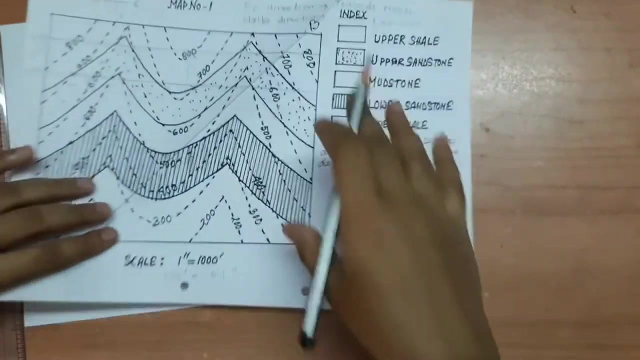 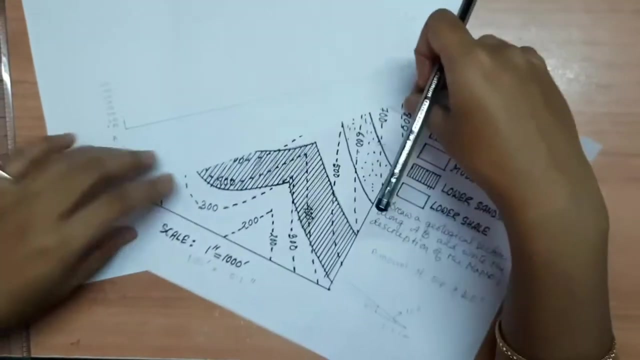 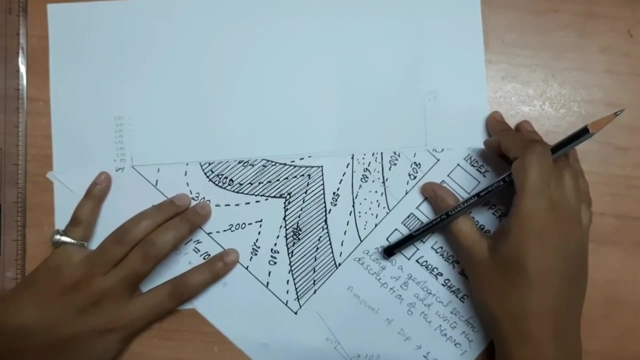 okay, So A and B. Now these are the contour lines and these continuous lines are wedding plans. we know that. okay, Now transfer this contour lines, contour lines and wedding plans from this map to this page, this graph: okay, So this is the contour line, contour lines and wedding. 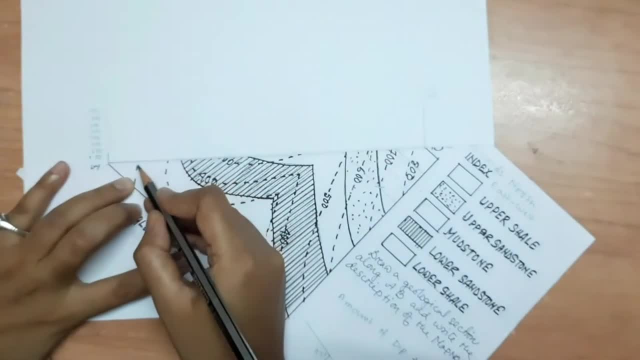 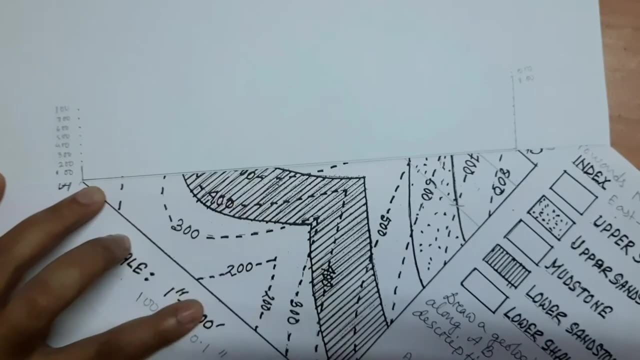 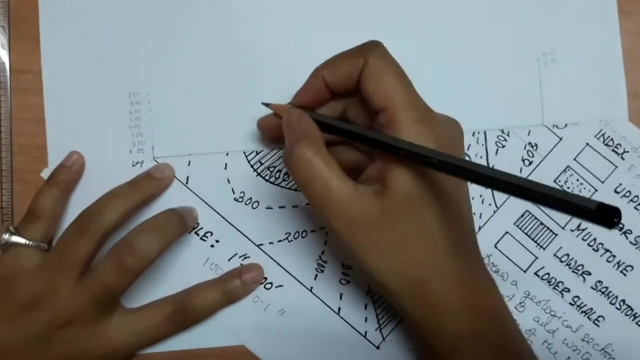 plans. So this is point A. point B: This is a contour line. first contour line, okay, Mark it as a single dot. This is again, and value of this contour line is 200, okay, So this is. 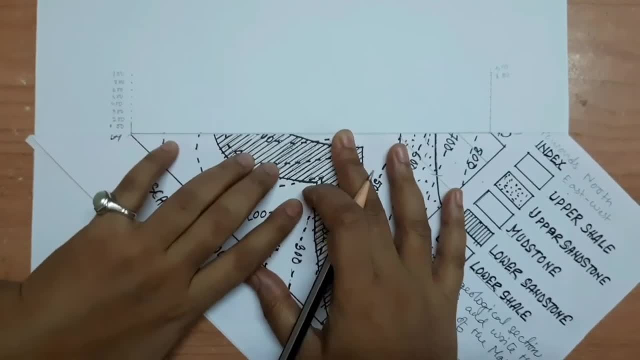 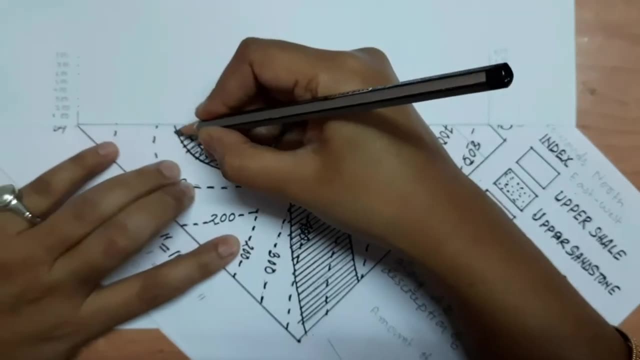 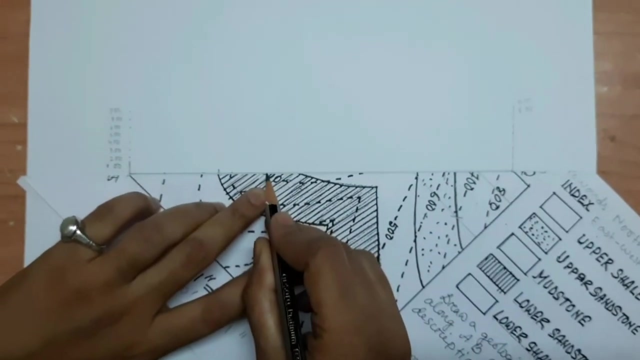 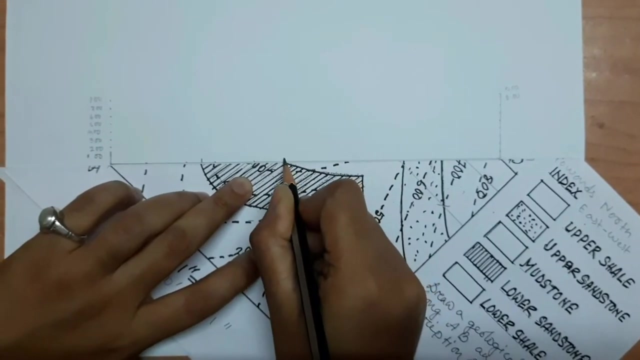 again another contour line. This is again another contour line. Contour line. this is a contour line and this is a bedding plan. Mark it as a straight line. okay, So this is again a. this is a contour line. okay, Again, dot. This is a bedding plan. This is. 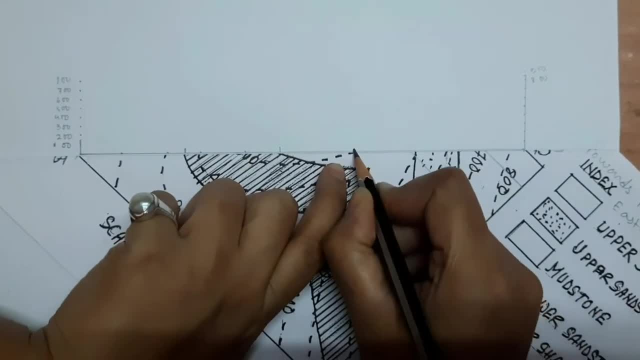 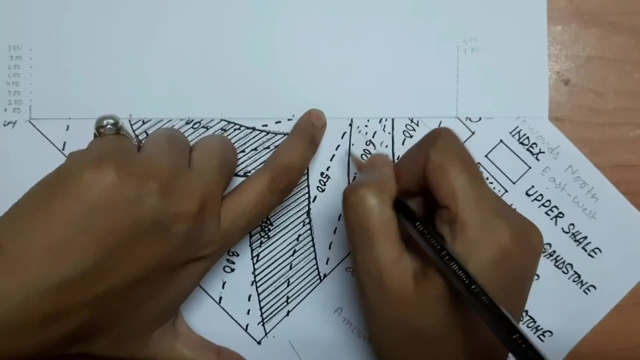 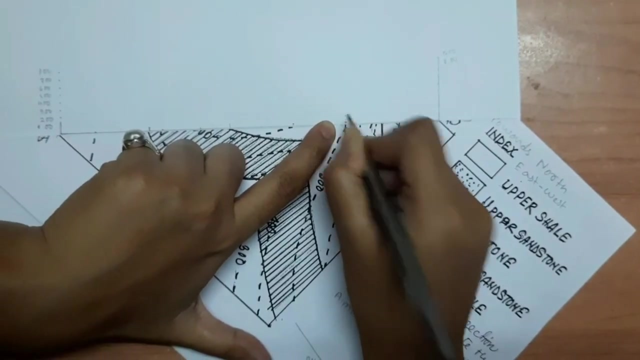 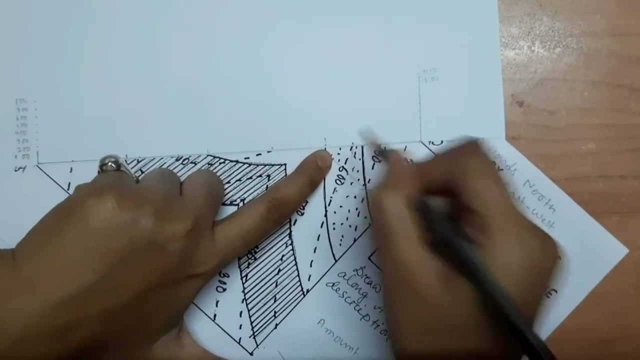 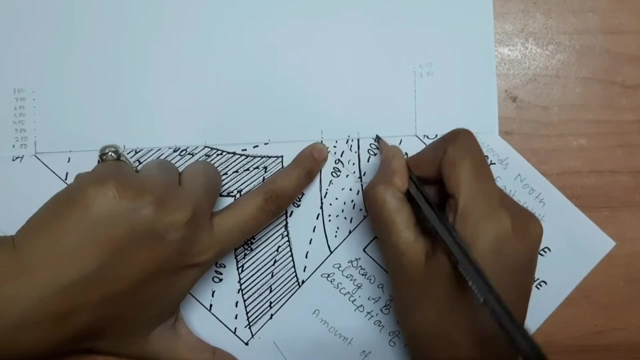 a bedding plan. This is again a dot, a contour line. Here there are both contour lines and wedding plans are there And this is a bedding plan. So this is again a dot a. So 1 dot and 1 leading plane. This is again a contour line. This is a leading plane. This is a contour line and this is your B point B. 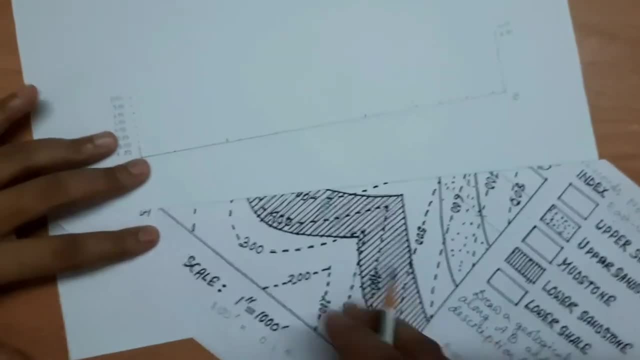 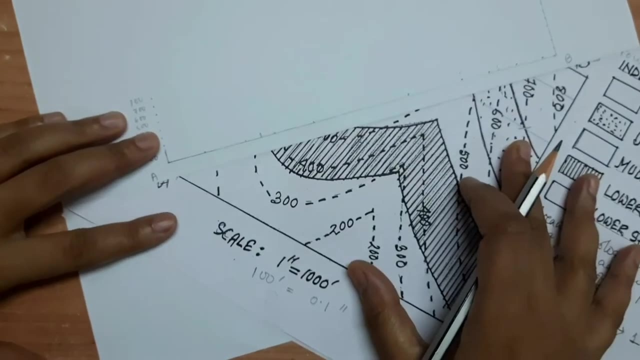 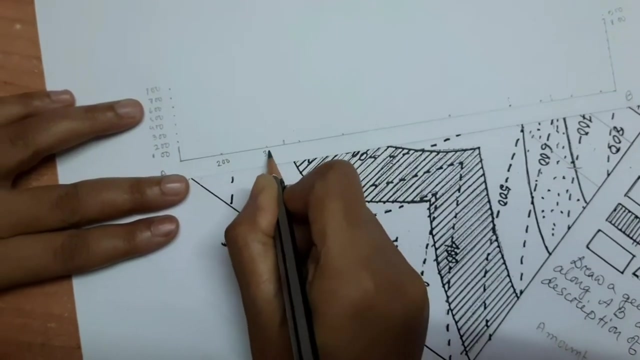 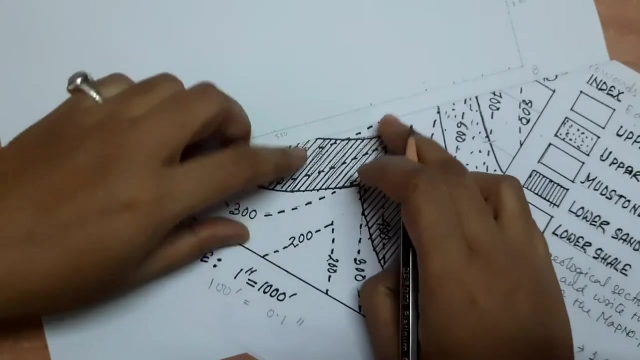 Okay Now, value of this contour line is 200.. Okay, So value of this contour line is 200.. Value of this contour line is 300.. This is 400.. 500.. This is again. value of this contour line is 500. 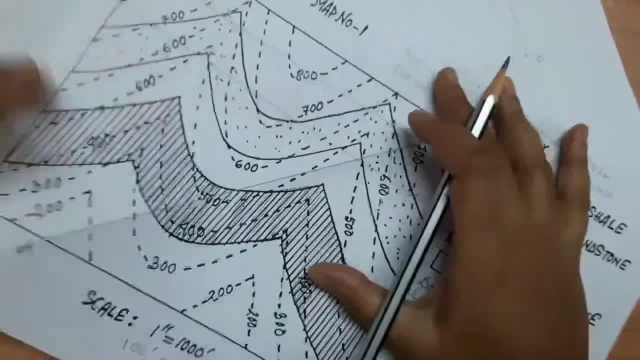 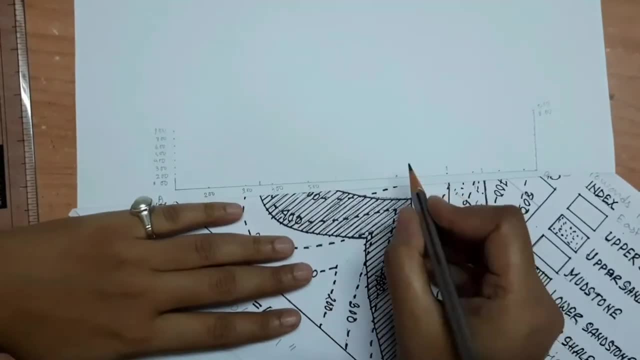 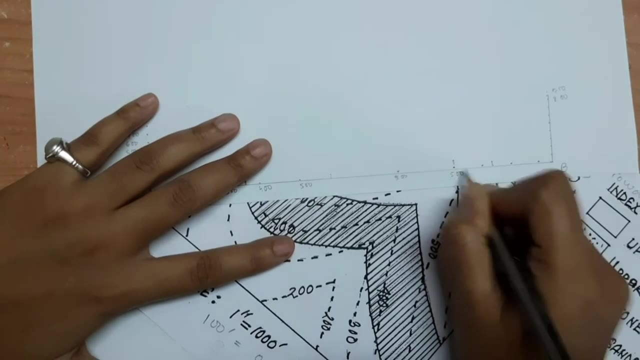 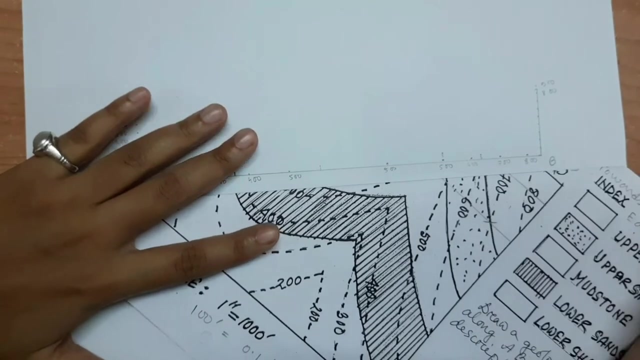 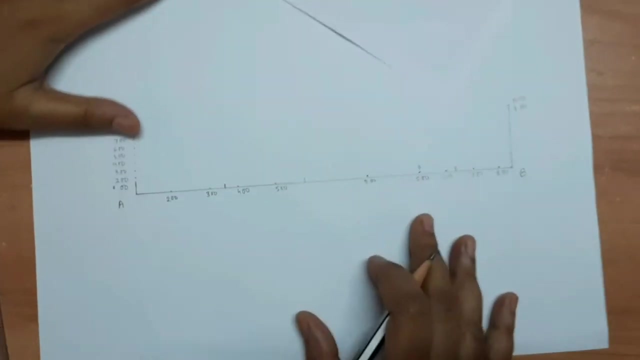 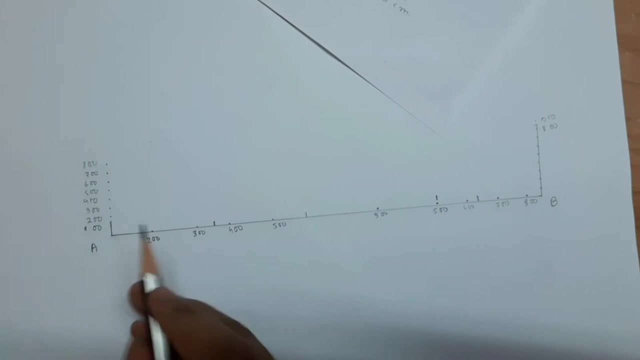 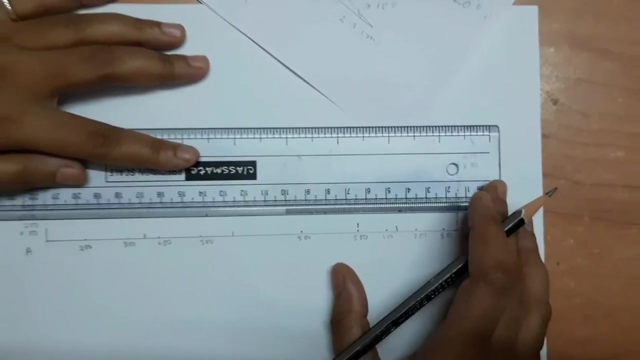 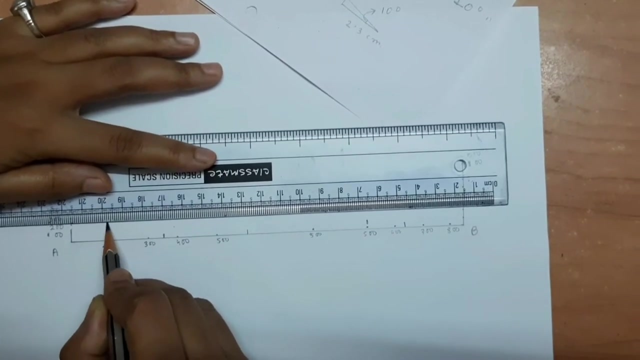 Okay, This is again of 500 contour line. Value of this contour line is again 500.. This is again 500.. 600.. 700. And 800.. Okay, Now, Now This 200.. Okay, This 200 means you are vertically. 200 means this point. Okay, This point. 300 means. 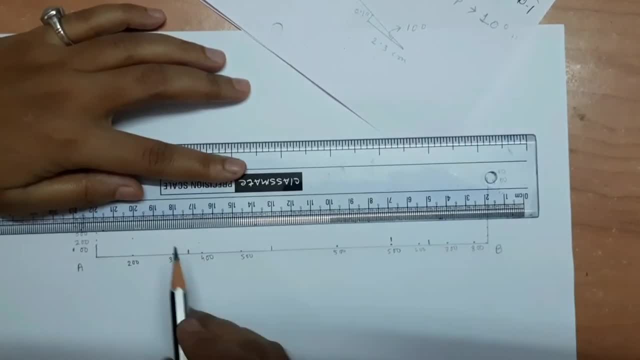 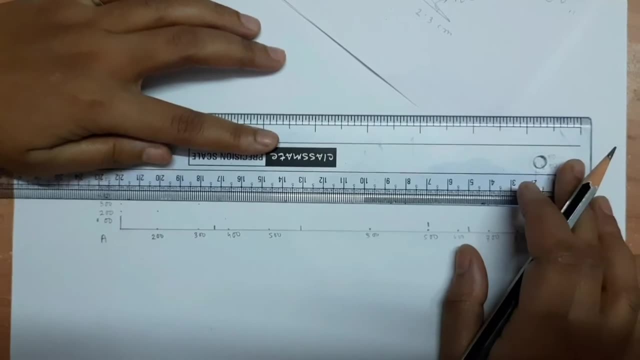 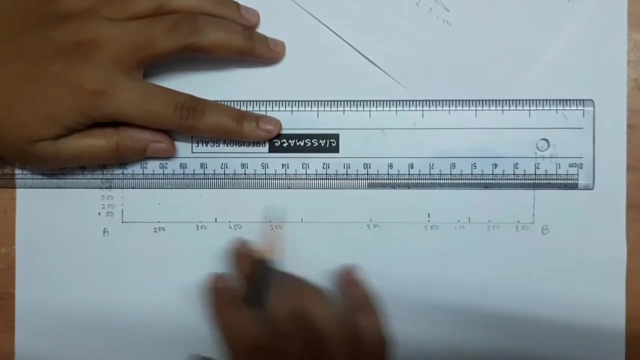 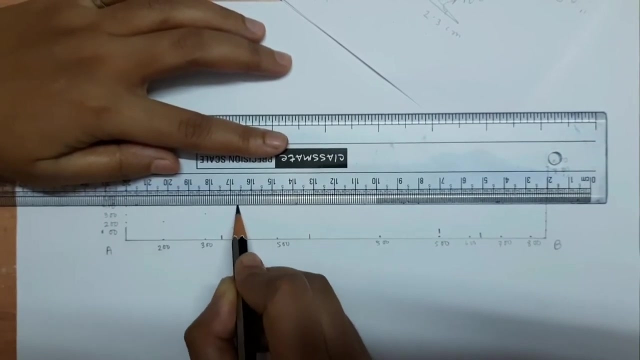 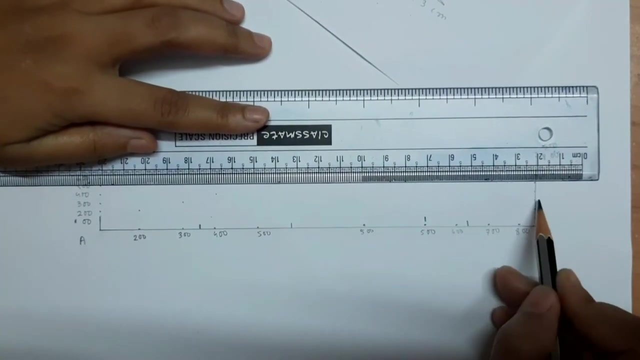 This point 400.. Just vertically transfer the contour lines. 400 means this is your 400.. 500.. Just vertically transfer the contour line. Okay, This point 300.. Just vertically transfer the contour line 500- 500. 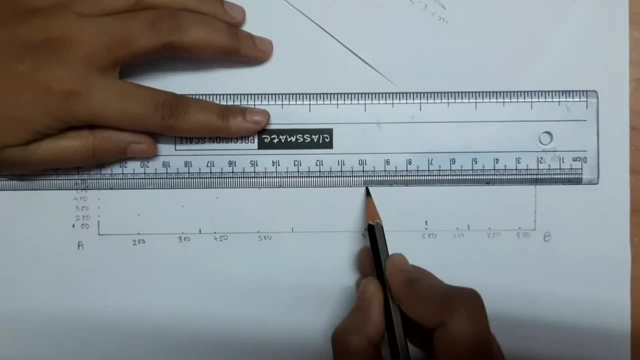 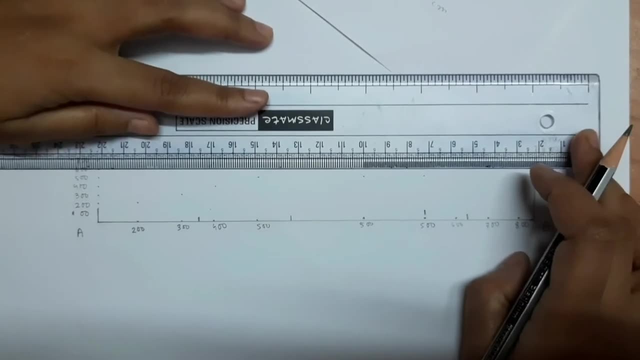 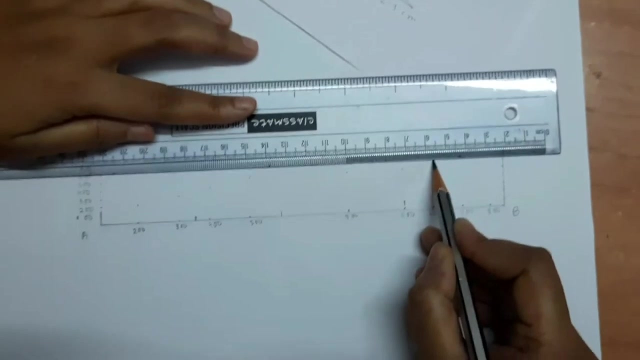 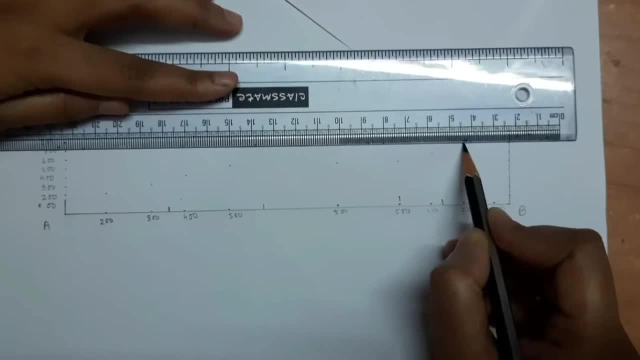 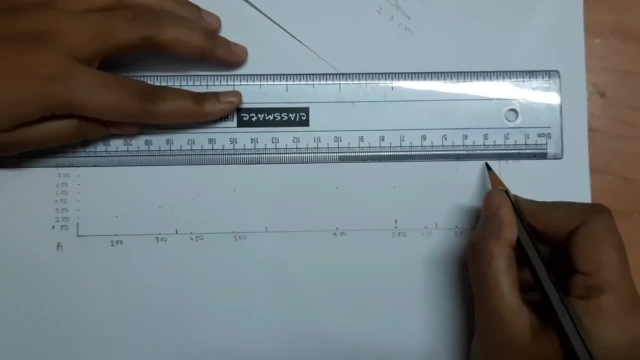 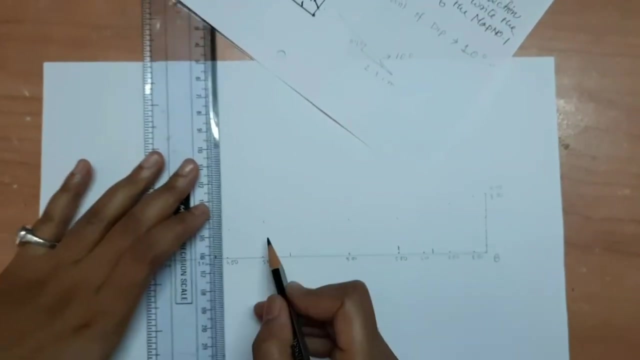 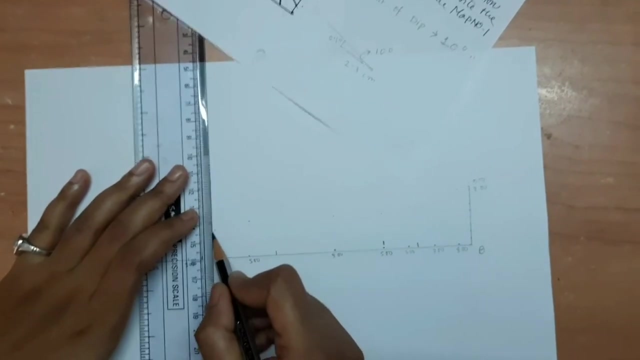 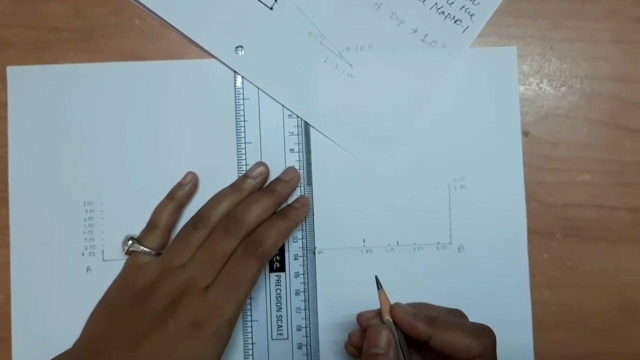 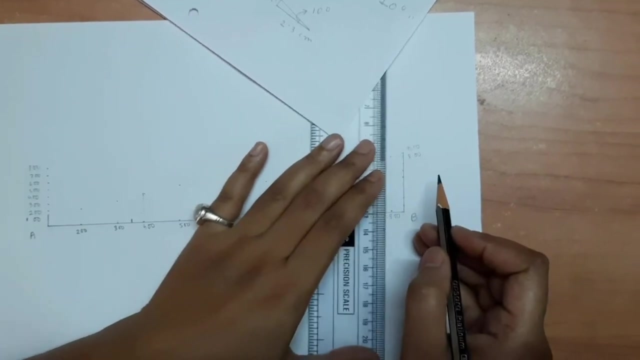 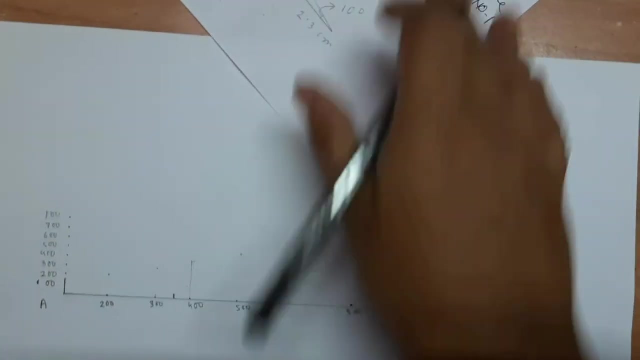 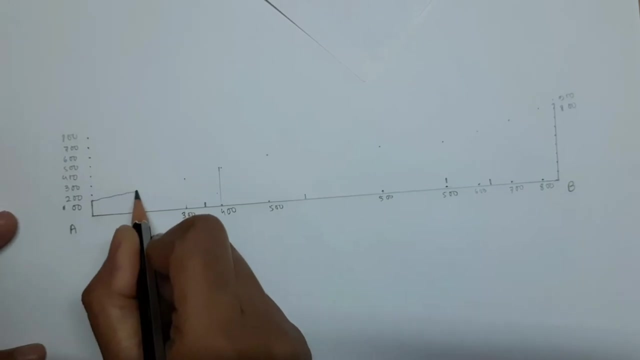 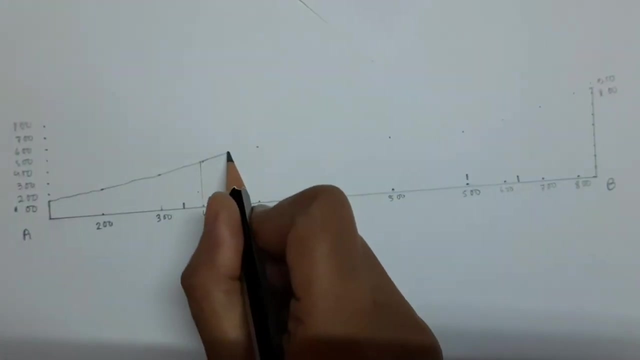 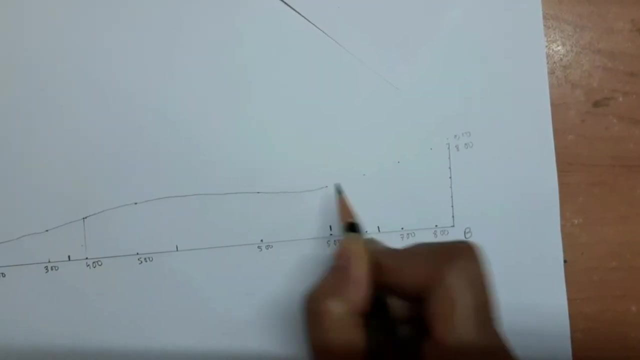 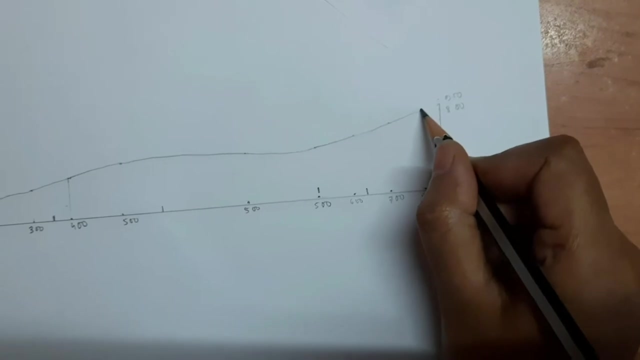 Then 700.. and this is 800. contour line 800. okay, just vertically, vertically transfer the contour lines, point. ok. okay, now join this point free and join this point. a point is this: So this is 200, 300, 400, 500, 500, 500, 600, 700,, 800 and this is your point. 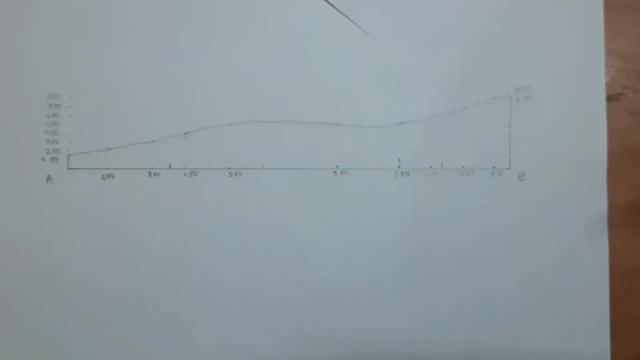 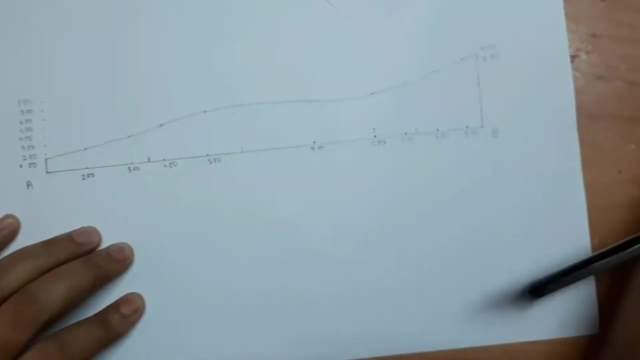 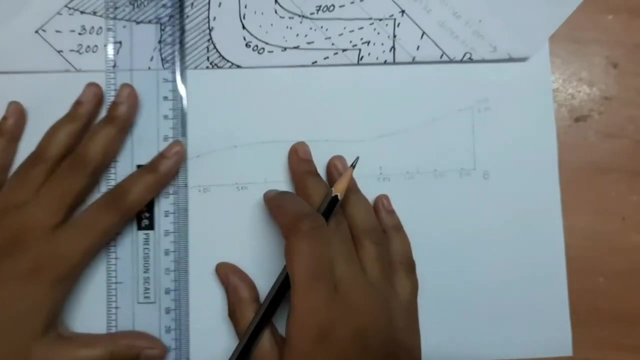 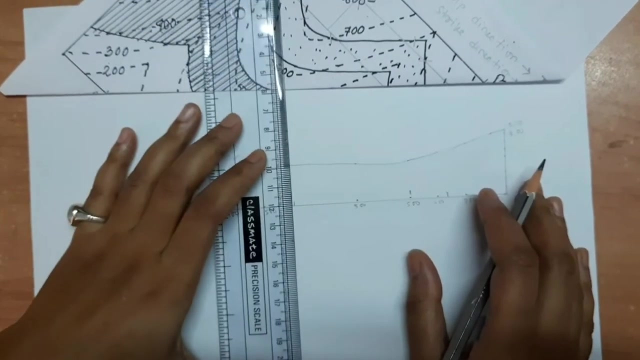 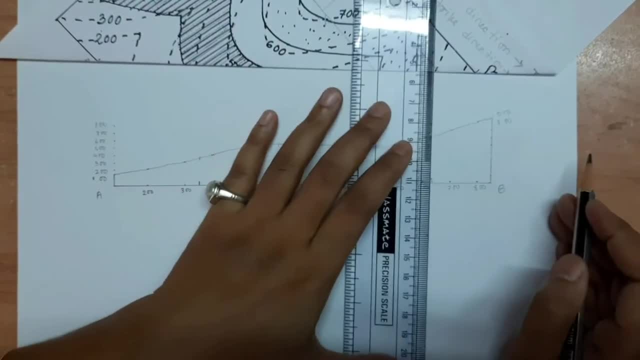 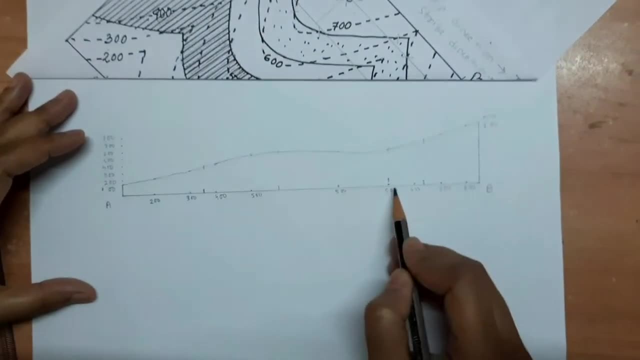 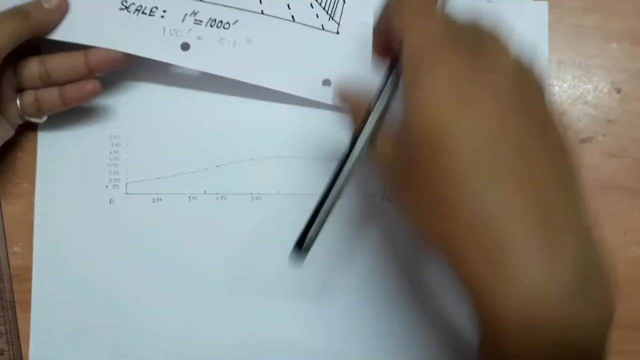 Radically transferred. This is a bedding plan, Again a bedding plan. Okay, So there are 1,, 2,, 3, 4 bedding plans, 4 bedding plans. Okay, Now how to draw the bedding plans. 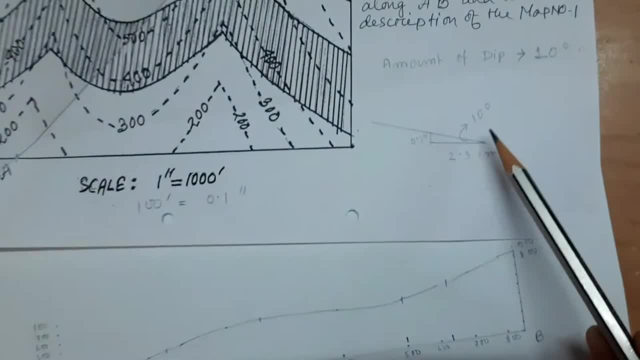 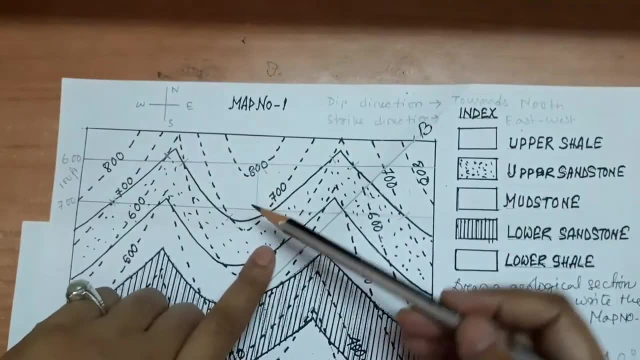 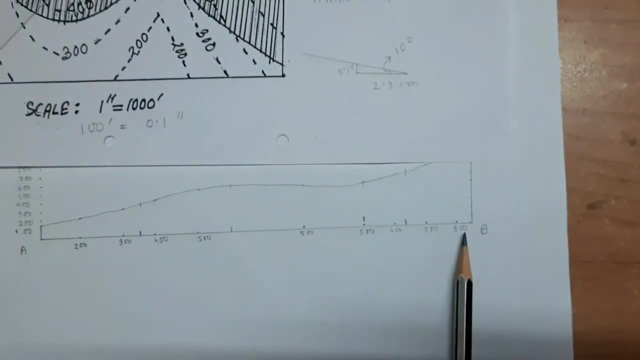 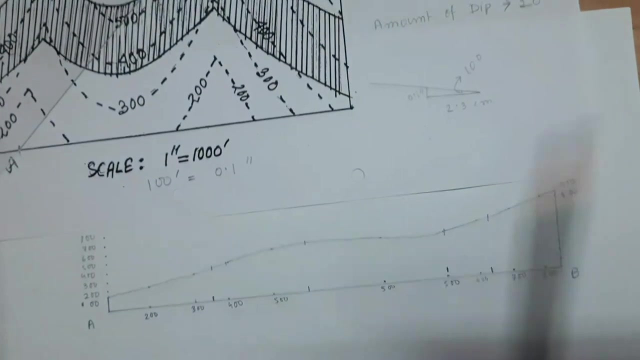 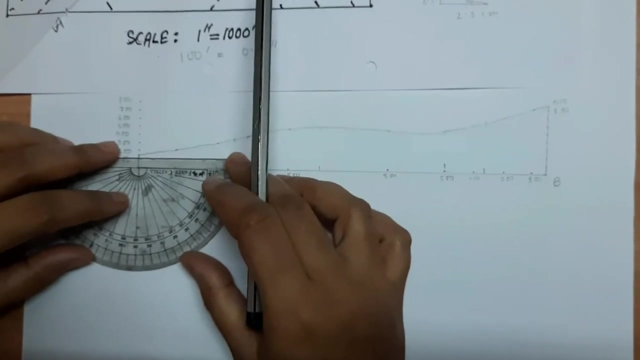 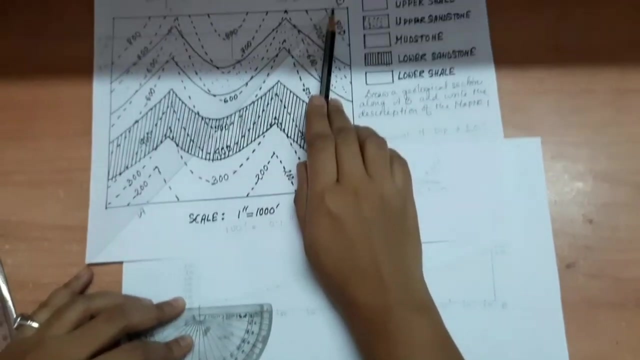 Now, your angle is 10 degree, Okay, Angle is 10 degree and dip direction is towards towards north. Okay, Dip direction was our dip direction. Direction was towards north, Towards. north means towards B, Towards this point. Okay, Deep direction is towards this point and deep angle is 10 degree. Okay, So this draw the 10 degree angle from A point because our direction is towards B, Towards B. Okay, Direction is towards B. 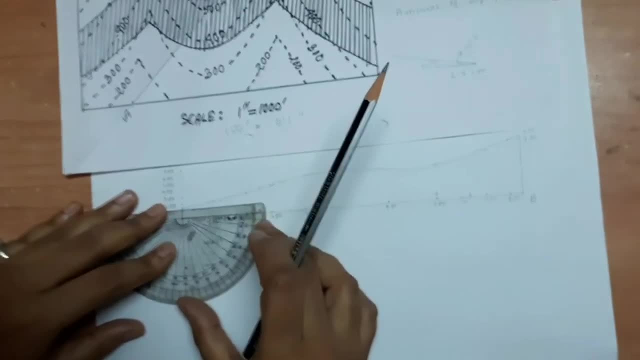 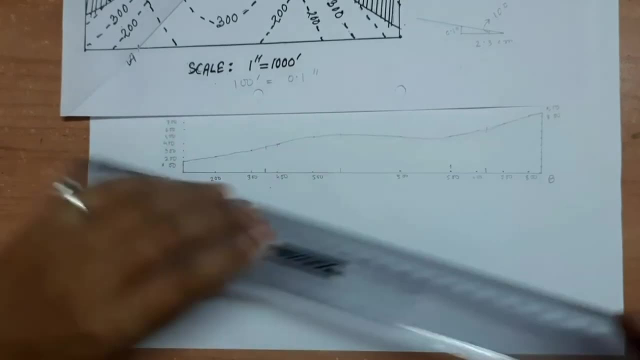 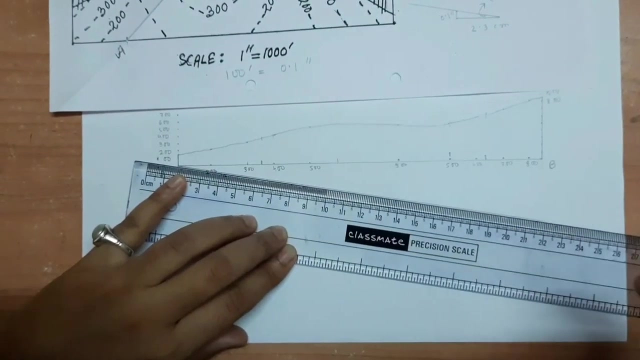 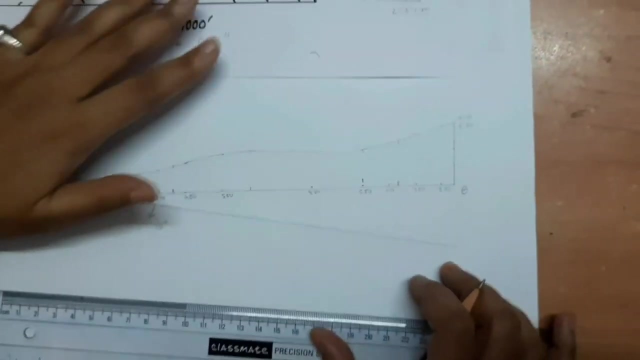 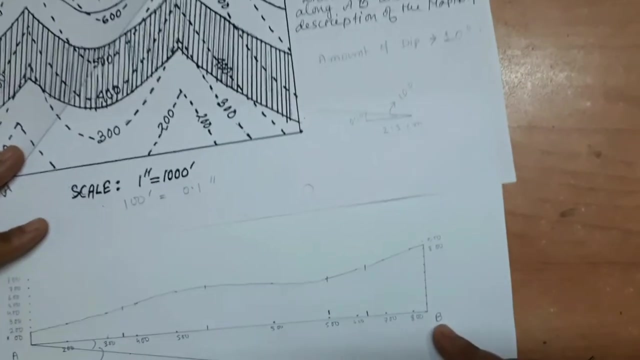 Okay, So here we have to draw the angle. So this is 10 degree, Okay. Okay, Now that means deep angle is 10 degree means and deep direction is towards B. That means why your bedding plans are inclined towards that direction. Okay, 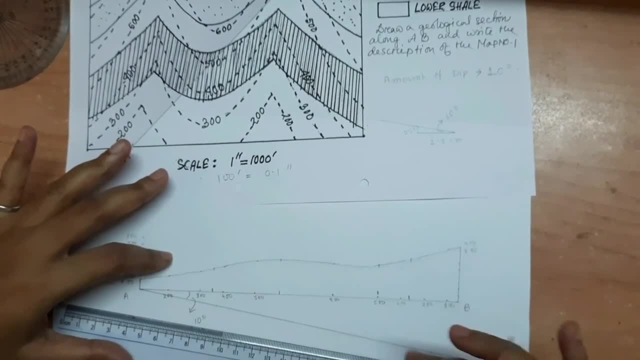 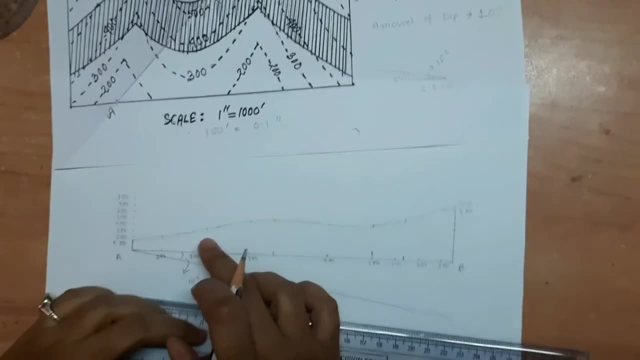 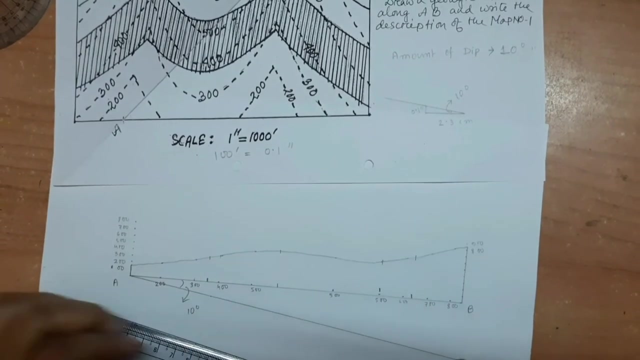 That means these are our bedding plans, and these bedding plans are inclined towards B, Point B, Or inclined towards north. So this is your first bedding plan. Just parallelly, draw the bedding plans, Consider this line and parallel, Make parallel With this line. 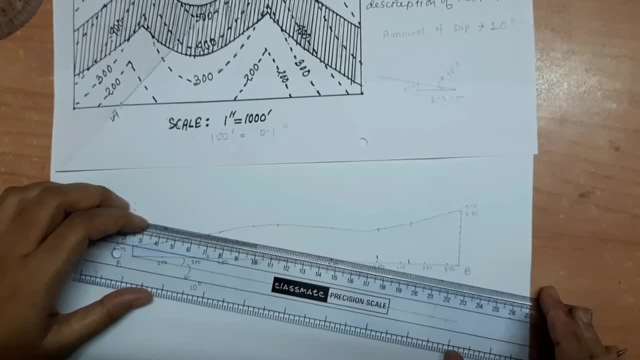 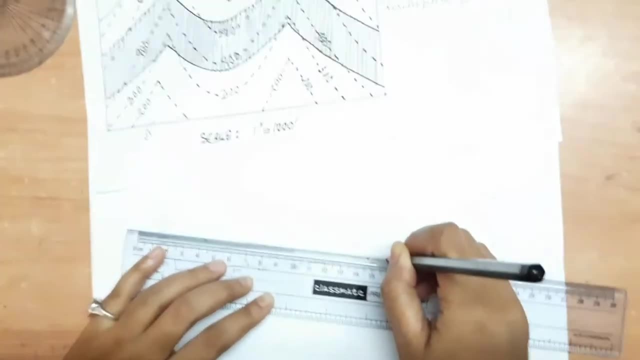 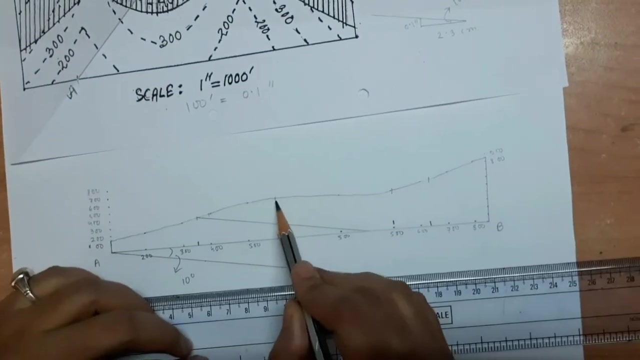 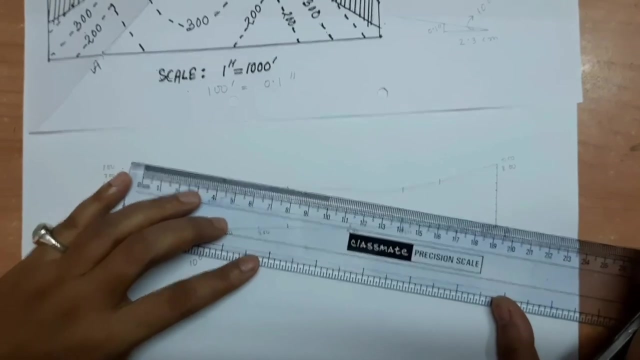 So this is our first bedding plan. Okay, Then for the next bedding plan. this is the bedding plan From this point, only From the topographic level. this point, Not from this point. Okay, Okay, Okay, Okay. 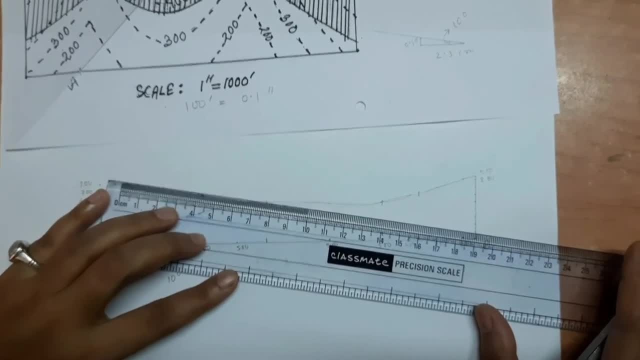 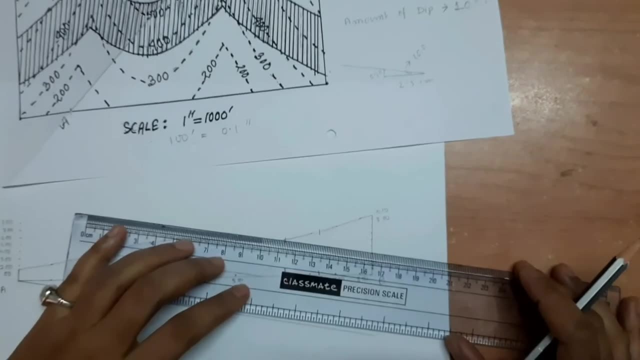 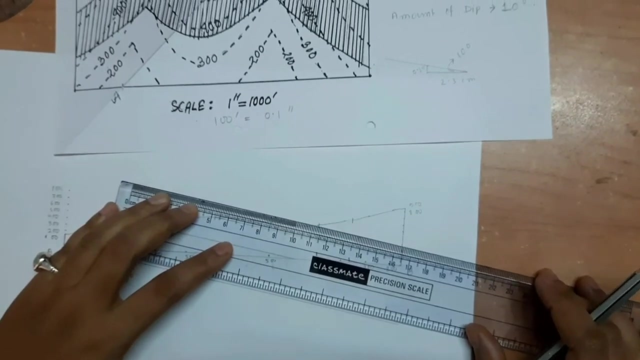 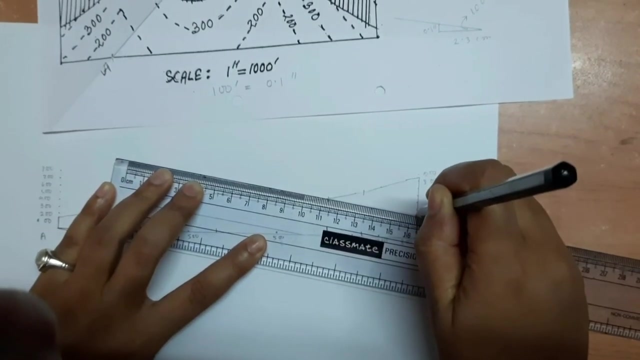 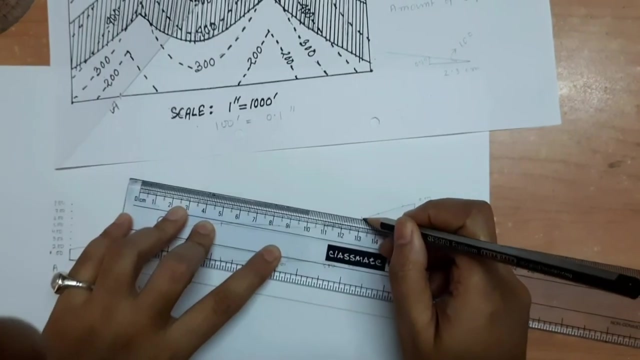 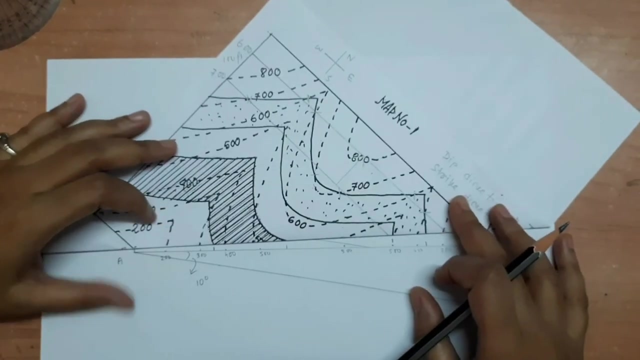 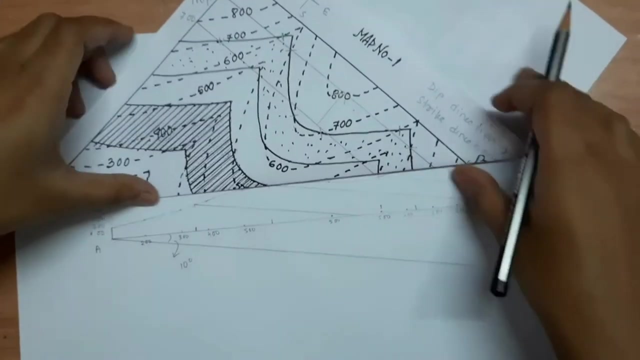 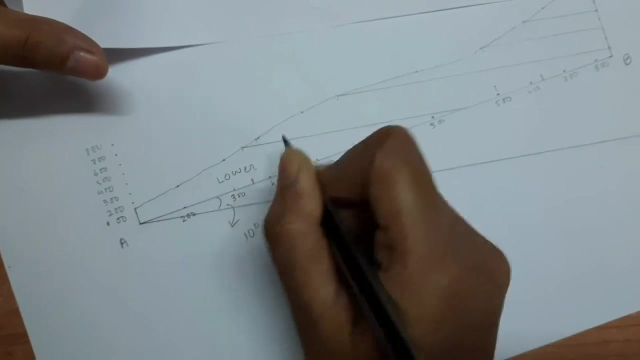 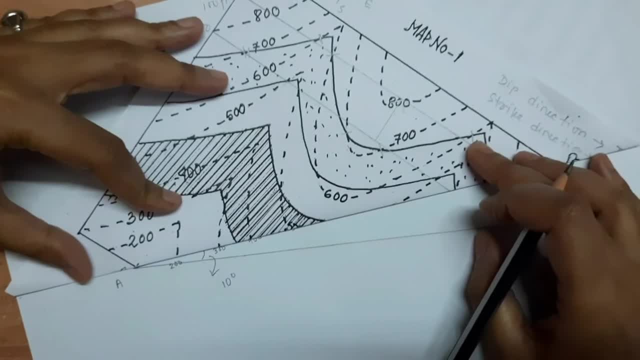 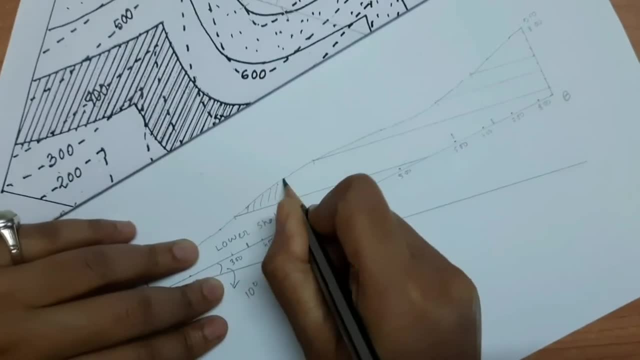 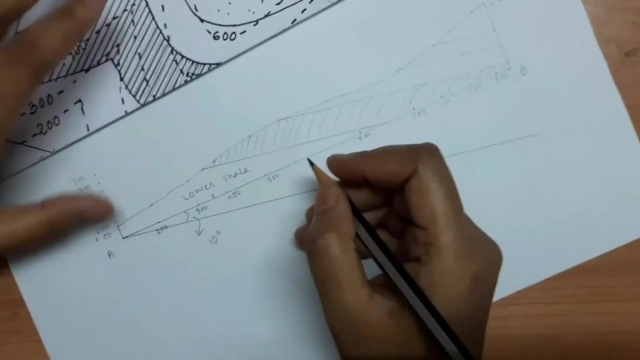 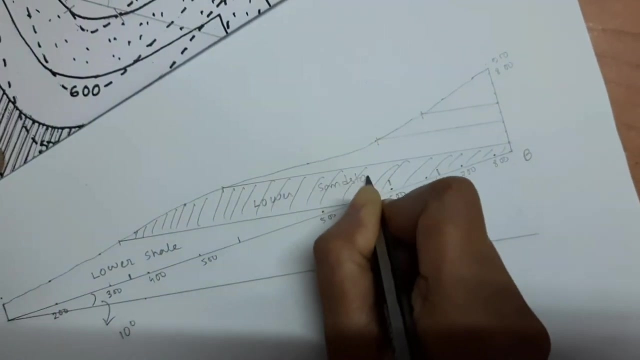 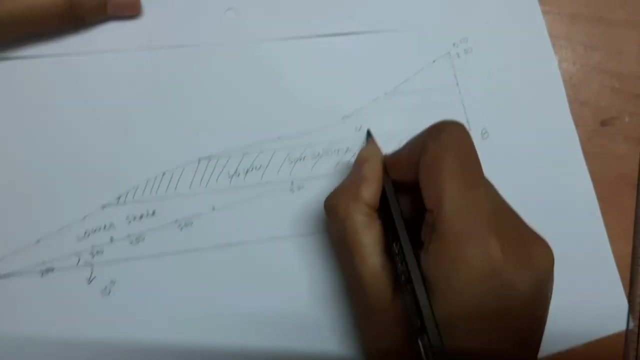 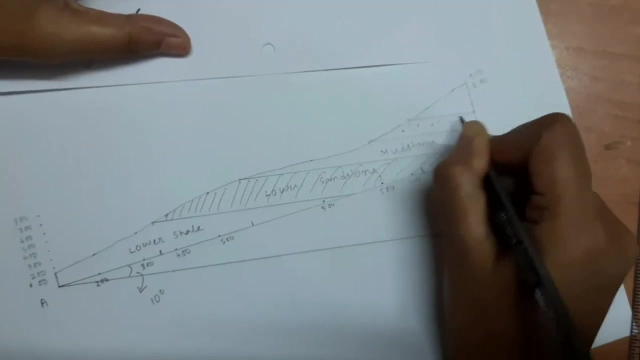 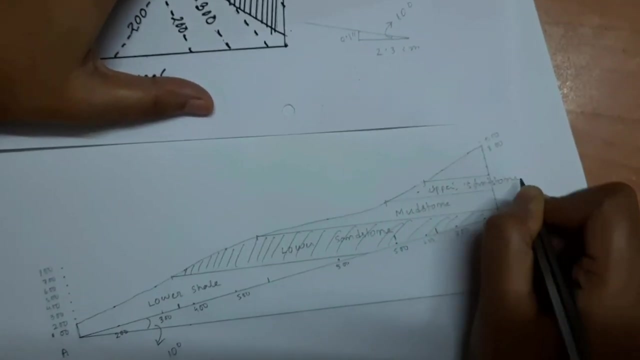 You can compare it here. This is the. That means this: This is lower sandstone, Lower sandstone, Then this one is lower sandstone. This is the mudstone, This is upper sandstone, Upper sandstone and upper shell. 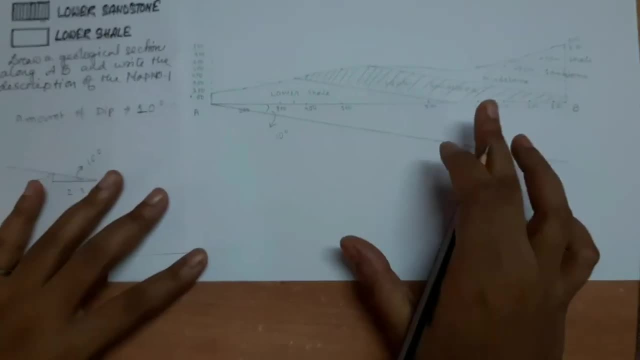 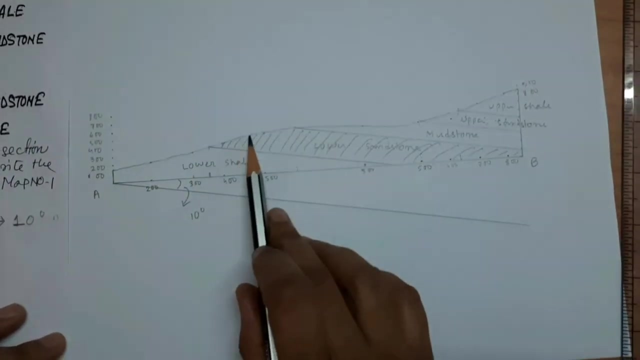 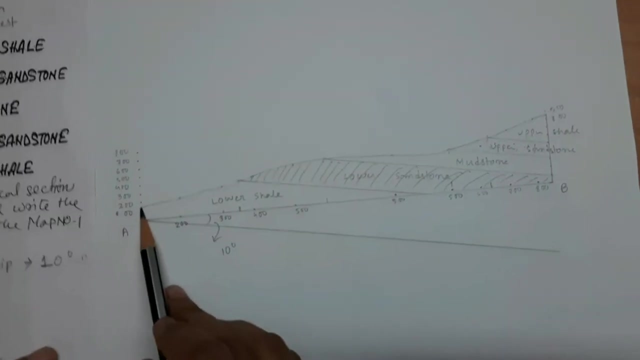 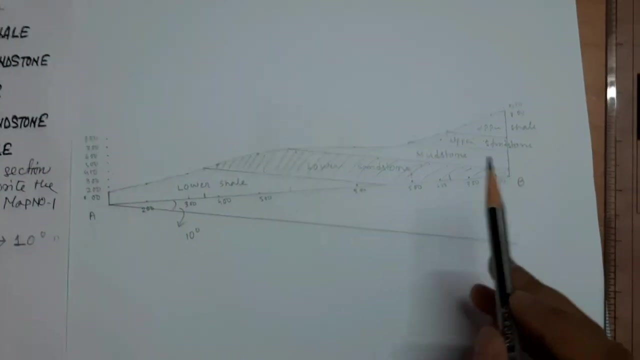 So this is your geological section? Okay, So here in this section, there is a hill, Hill. All type of structures are there. One valley is there. One half exposed valley is there. Again, one half exposed hill is there. Okay, In this topography, In this geological section.